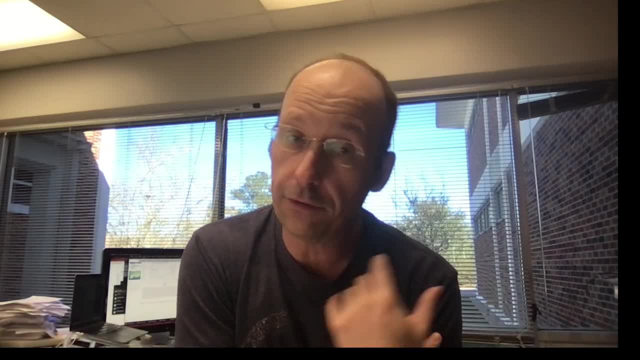 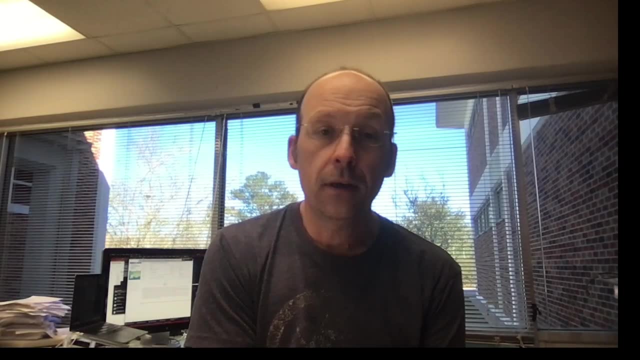 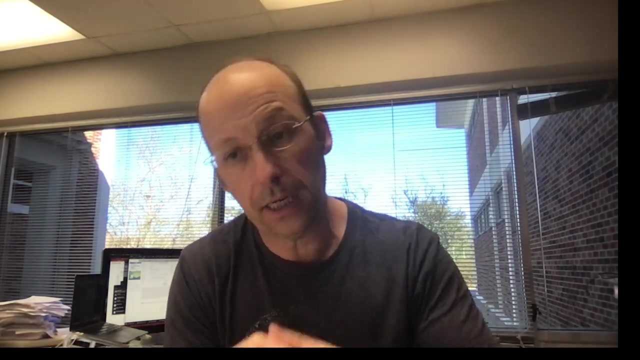 situations where work energy is much better And there's some things that work energy doesn't do well. So you got you have both of those and I left my window open for you today. Hope you like that. So work energy, Oh, the other thing is most textbooks, including this, one kind of break up work. 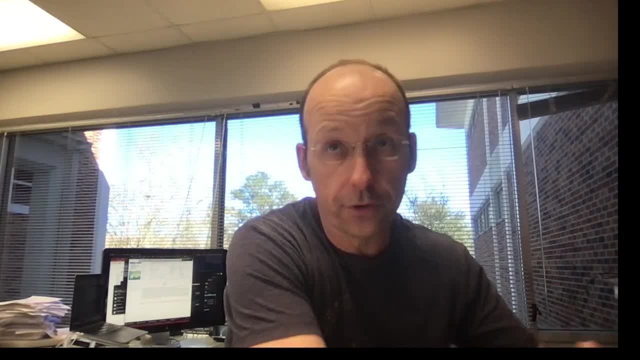 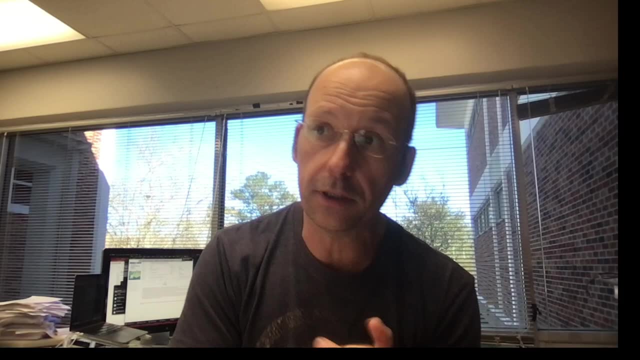 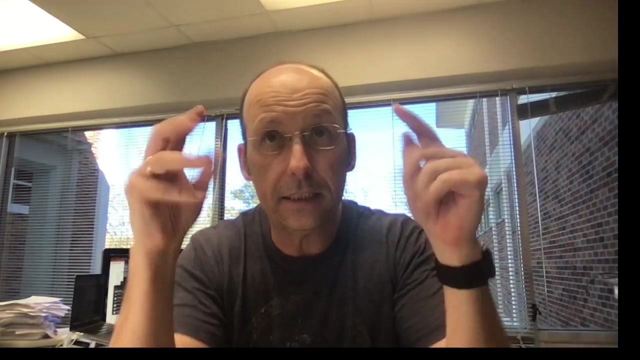 energy in terms of first looking at work energy and then looking at potential energy. So I'm going to follow along with the book. I'm going to talk about a couple things that the book doesn't talk about, but I'm just going to do that. And again, my whole playlist is down below in the in the 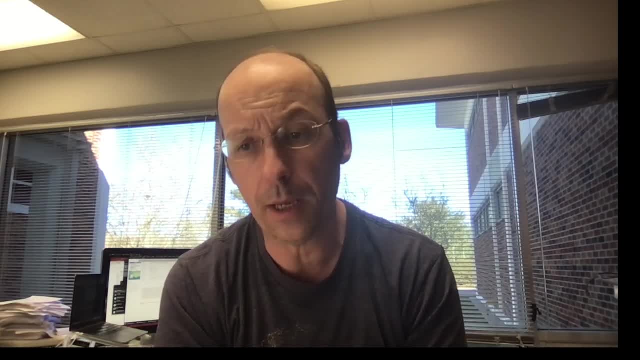 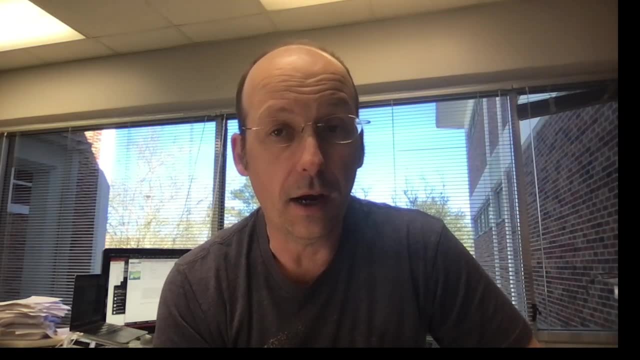 description And I'm not really going to work examples. If you want examples, you can just ask, and I can either. I have one already. you can search in the, in the search thing up there, wherever it is. But I'm just trying to get the summary, just just the main idea. Okay, so let's. 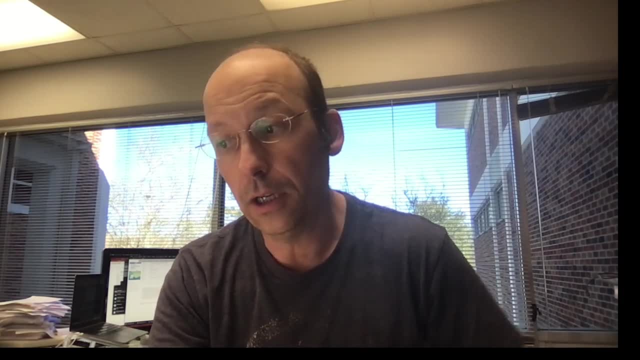 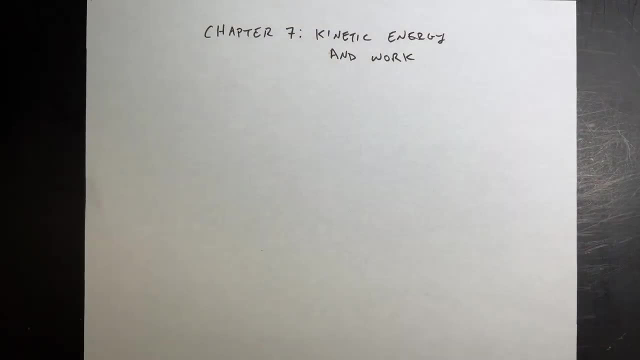 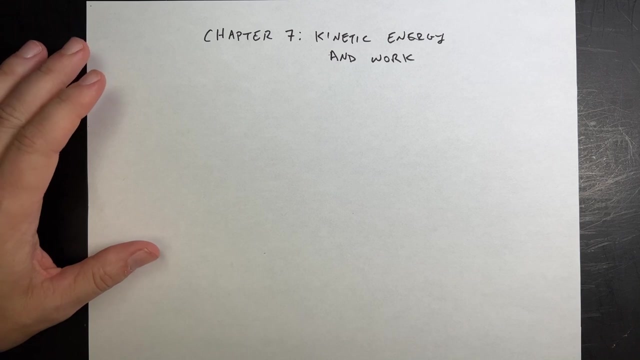 jump into it. I'm going to switch over to the paper and we can start talking about chapter seven: kinetic energy and work. Okay, so here we are, Chapter seven, kinetic energy, work. That's so, let's start off. I already talked about energy. Let's talk about kinetic energy. So, if I have a 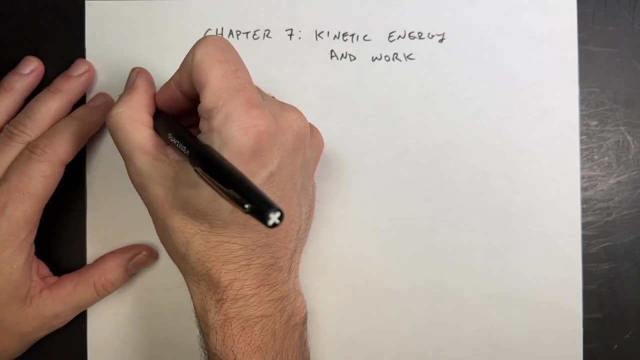 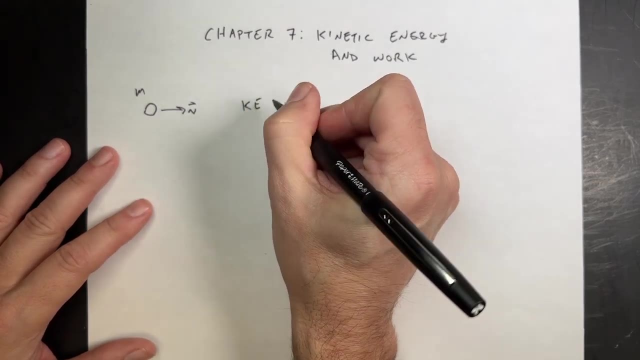 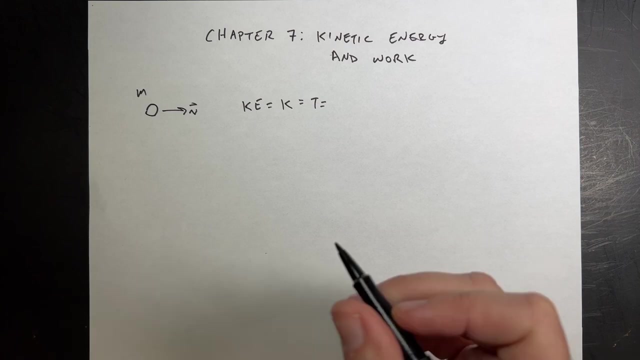 ball and that ball is moving with some velocity v and it has a mass m. Well, we can associate an energy with its motion and we call that kinetic energy And a lot of times people write it as ke. Sometimes they write it as k. In classical mechanics we write that as t, But it's all the. 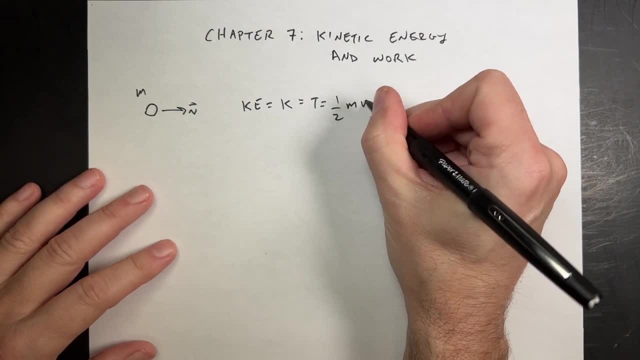 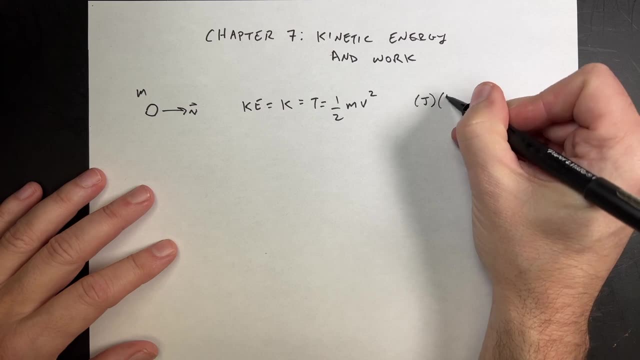 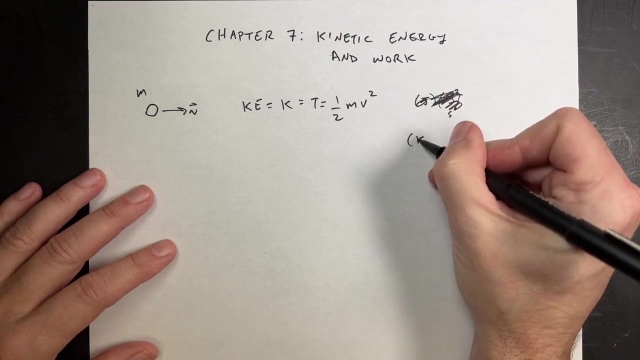 same. We can calculate that as one half m v squared. So if you have that energy you can write the mass in joules. So if I have one joule times meters squared per second, I said joules. That's not true. If you have kilograms and then meters squared per second squared, that's equal. 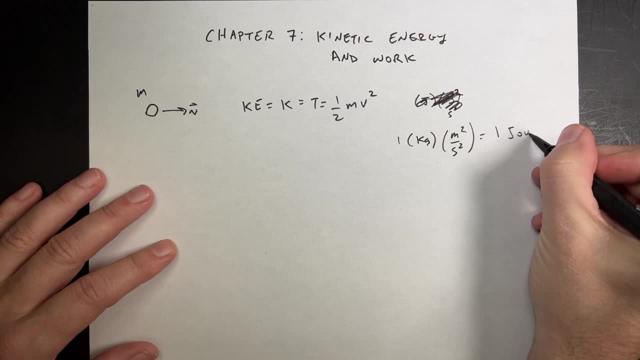 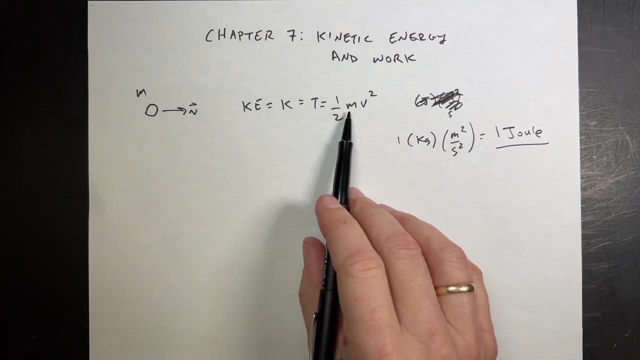 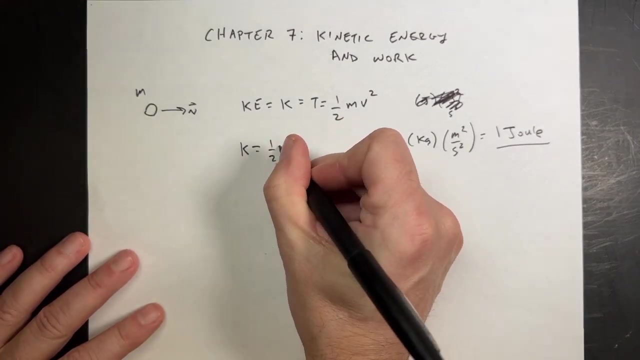 to the unit of one, One joule. So a joule is a unit of energy that we'll see. That's a j. One of the things also you need to know about this kinetic energy is that velocity is a vector, So you might want to write this as k, as one half m magnitude of v squared, One of the 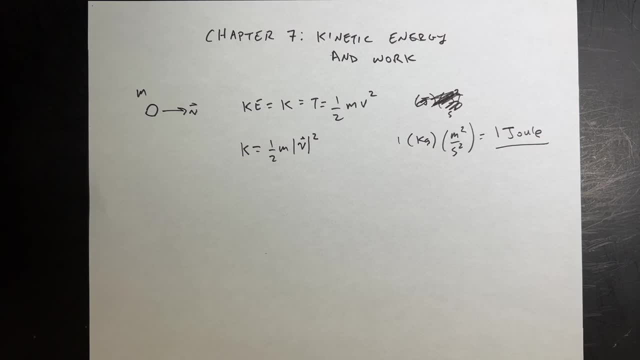 things we're going to really see is work and energy are both scalar values. They do not have a direction. You don't have a direction with the kinetic energy, It's just a value. It doesn't tell you which way you're moving, Just a property based on both the mass and the speed. Okay, what about? 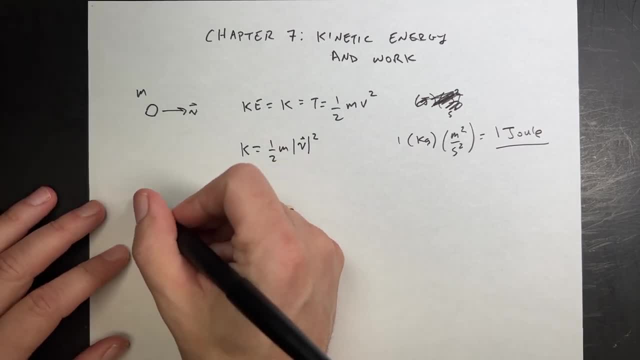 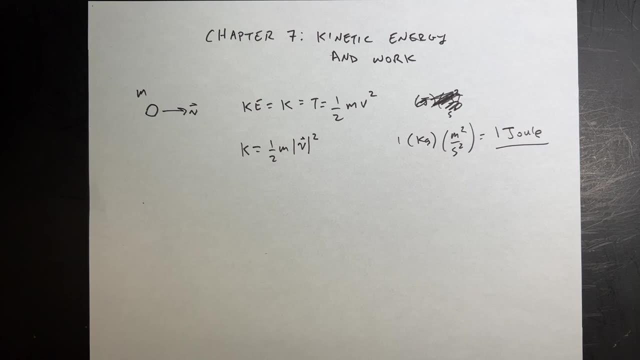 work. Now the book defines work as work. You can think of work as a way to add energy to a system, and it didn't really define systems too well, So I'll talk about systems too Well, let's do that. So suppose I have some imaginary grouping of stuff like that, stuff Who knows what it is, and I have 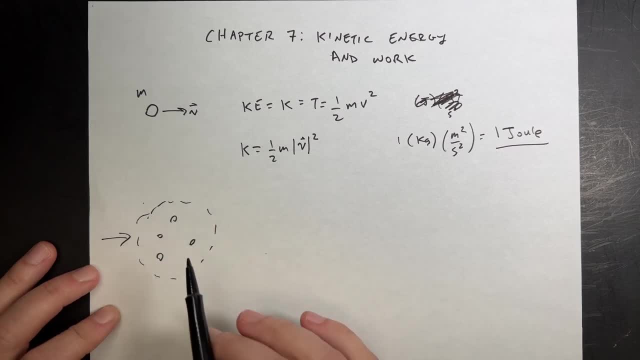 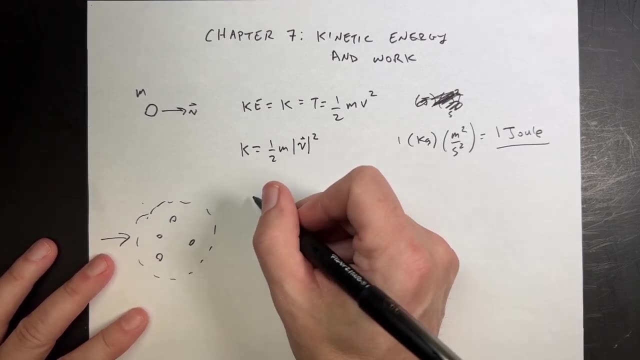 some energy input into the system. Well then, the energy of this whole thing is going to change. So one of the ways we can calculate the energy input is with work. So the book defines it as this. I'm looking at what it does, this Work done by a force One. 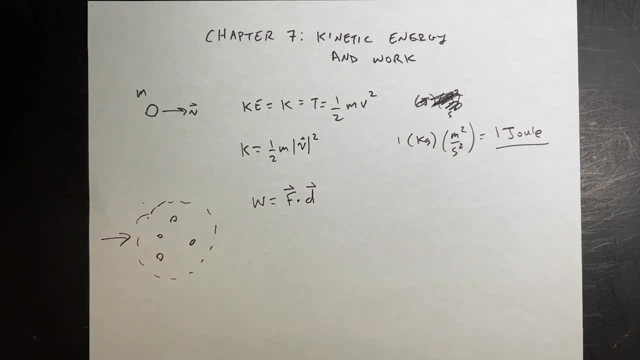 single force is F, dot D. Okay, where F is the vector force, D is the displacement and that's the dot product. We went over that in chapter two when we talked about vectors. No, chapter three, We talked about the dot product. I'm going to review it just in a second, just to remind you. I don't like that. 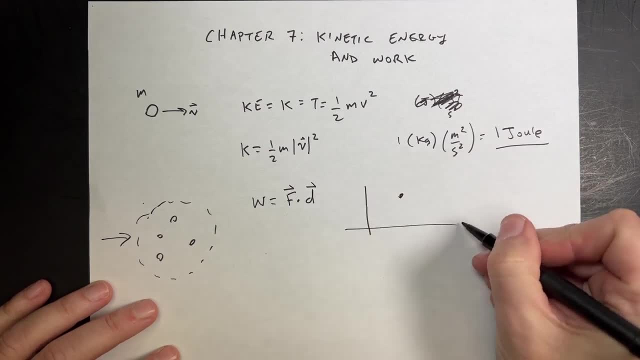 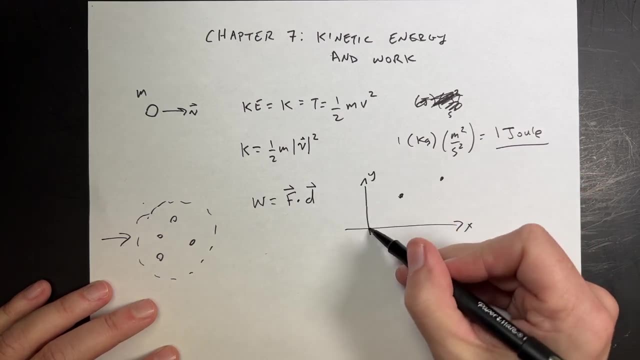 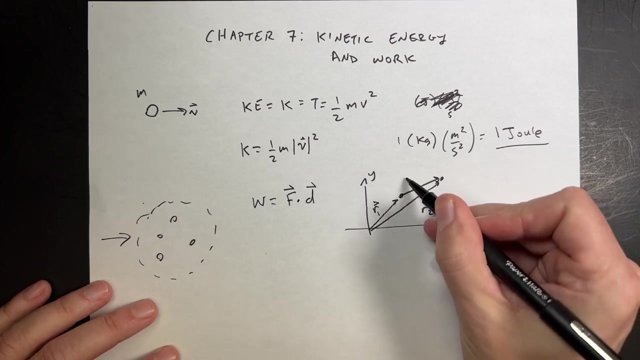 displacement Right. So if I have, let's say I have this, Here's my X axis, Here's my Y axis. I start here and I end there, So I could call this R1.. I could call this R2, and then I could call this vector delta R. 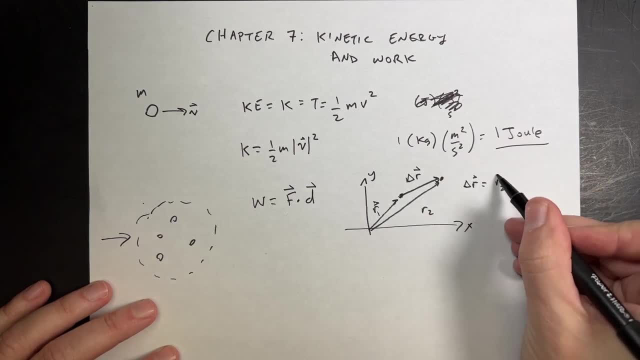 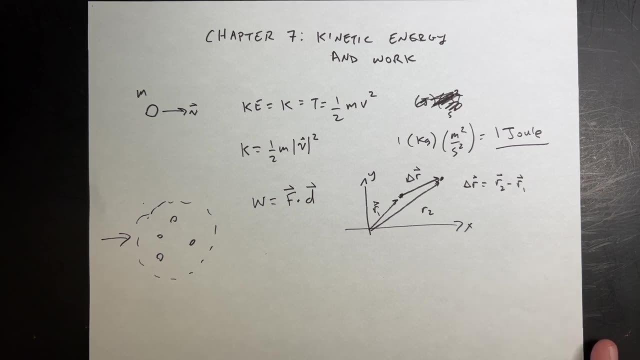 So delta R is R2 minus R1.. And that's, I think that's the better, more mature, more grown up way of writing the displacement, Because it incorporates all these things. Calling it D is is, I don't think, very, very useful, So I'm going to write work is F dot, delta R. I like it better that way. Now, this definition is only true if the force is. 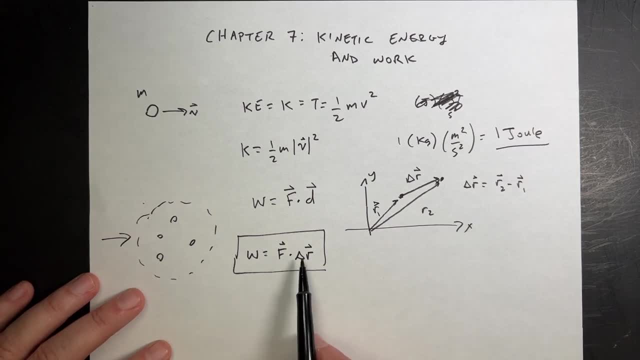 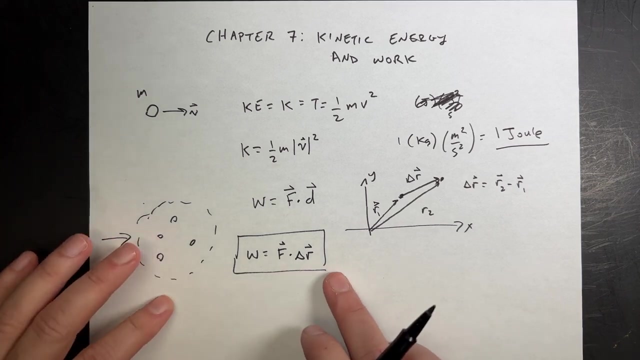 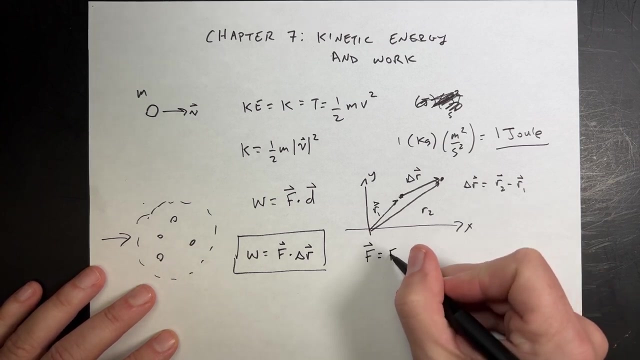 constant and the relationship between F and delta R is constant. So you can't have, like that, be a straight path. It can't be some swirly path, which which I'll talk about, but it's more difficult to calculate. OK, So let's review the dot product, because that's what this is. So if I suppose I write the force as a vector, I'm going to use the notation the book uses. 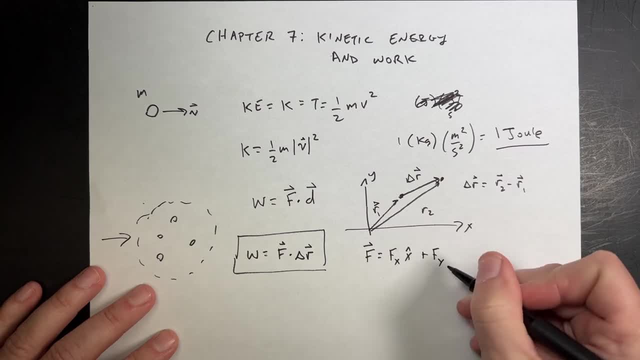 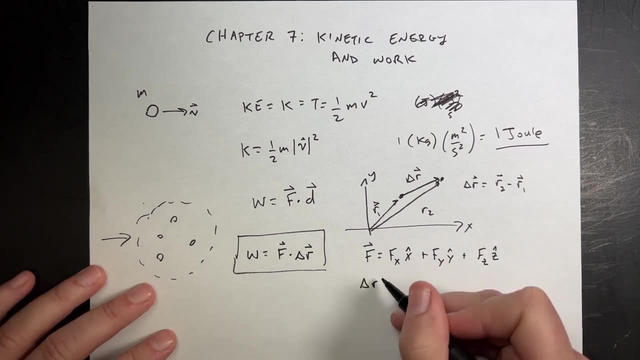 F X in the X direction, plus F Y in the Y direction, plus F Z in the Z direction, and then delta R. It's going to be equal to. I don't want to write delta a whole bunch of times, Let's write this as: 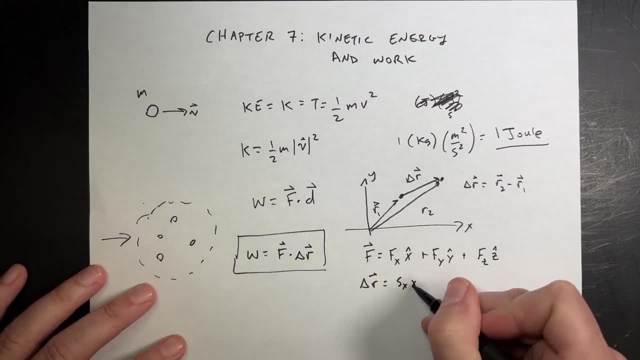 I'll call it S S, X, X hat plus S Y, Y hat plus S Z, Z hat. So these are, these could just be numbers, Number number, number, number, number, number, it could be OK. So if I want to take the dot product, here, 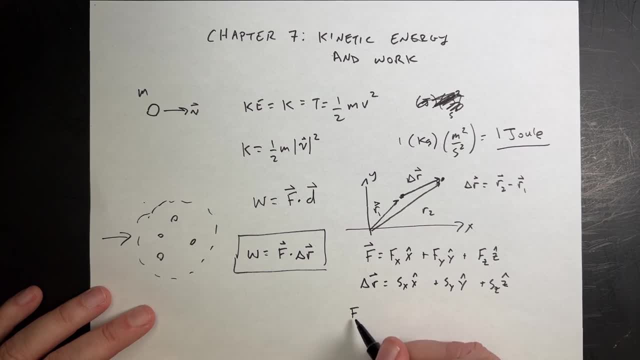 I could. the way to take a dot product F, dot delta R. You take the X components and multiply them together. You take the X components and multiply them together, OK, And then the Y components multiply together and the Z components multiply together and then you add them all up. 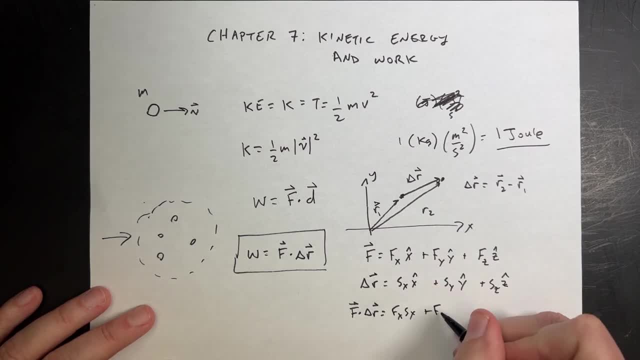 So it's going to be F X, S X plus F Y S Y, plus F Z S, Z, And so then you see that all these numbers are scalars, So you get a scalar value. Now there is another way to calculate this. Oh, I didn't get enough paper. 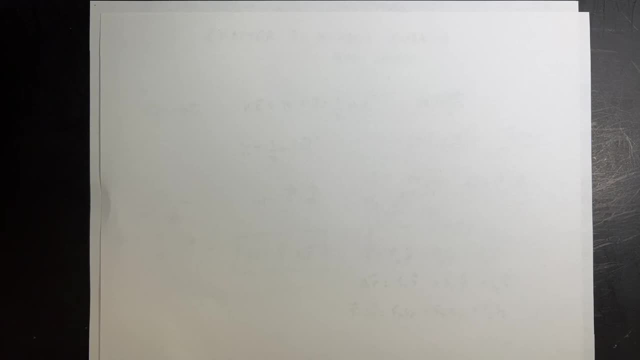 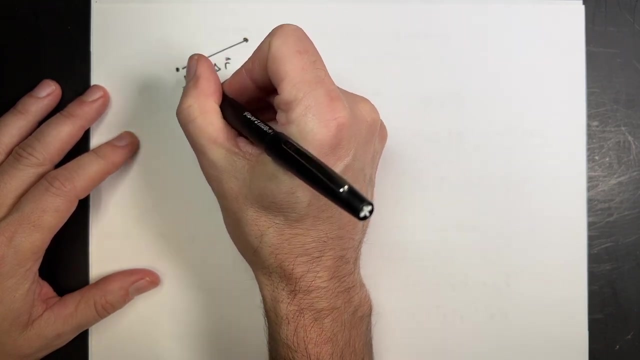 Let me get some more paper. I can tell This one is going to be a four sheet lecture at least. So suppose I have this. So that's my delta R, And then this is my force. I'll put it over here. 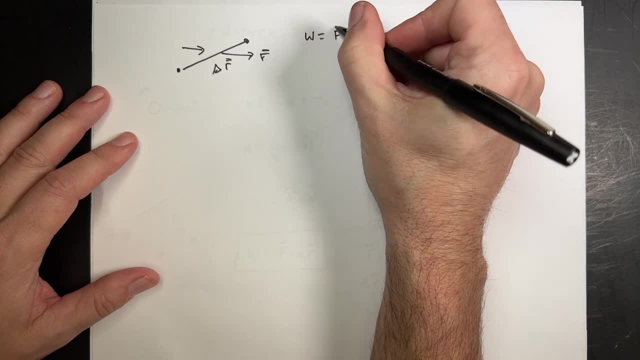 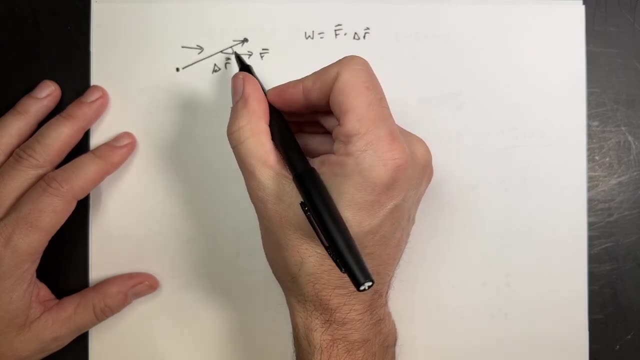 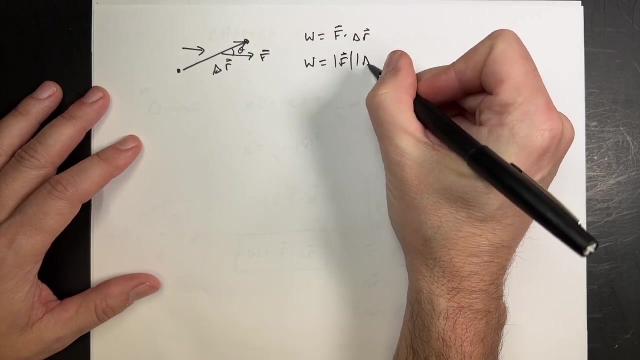 F, So I can do work is F, dot, delta R, Like I just did, But if I also know the angle, So this is the delta R, It's a vector. If I know the angle, theta between that, We can also write the dot product as the magnitude of F times the magnitude of delta R times the cosine of theta. 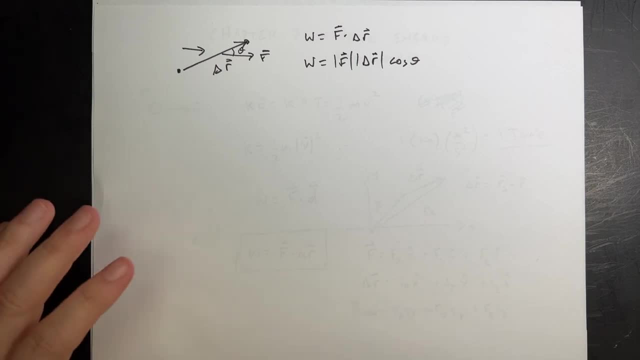 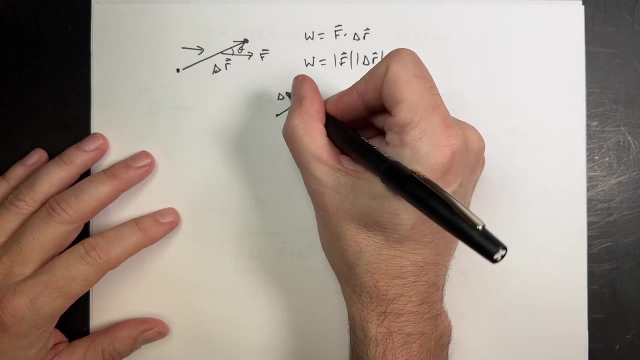 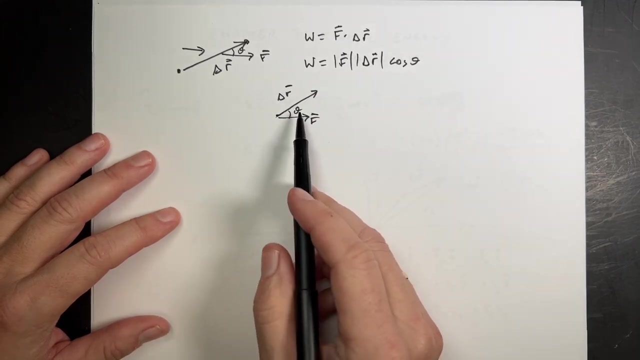 Now, in both of these situations you see something really useful. There's three situations. I'll just draw them out right here. So situation number one: I'll just write delta R and I'll say F and theta. So in this case theta is less than 90 degrees. 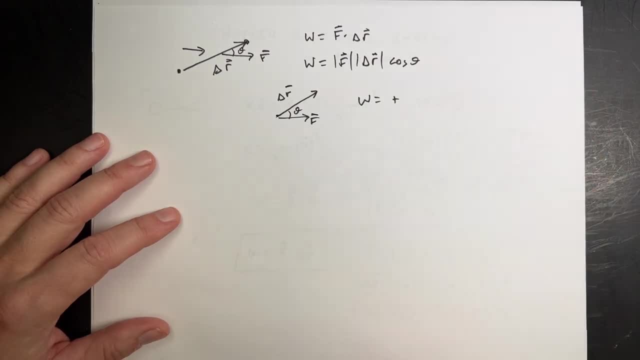 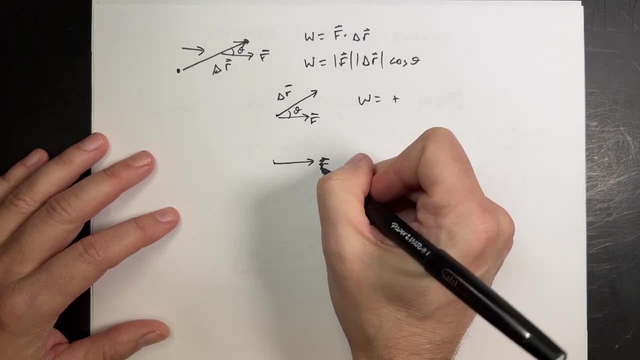 So the work done is going to be positive. Next, I could have this case F. Well, I want to call that delta R- I don't know why. I feel like I'm moving that way- And then F, And then that's a right angle. 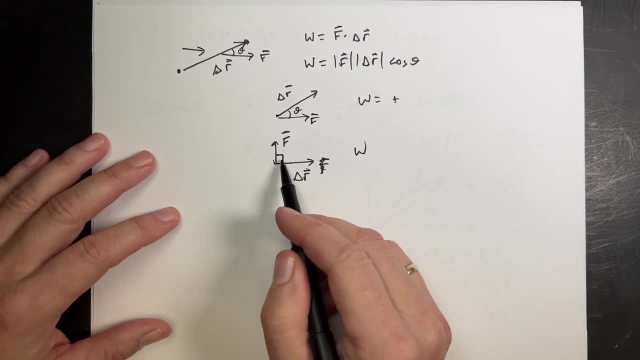 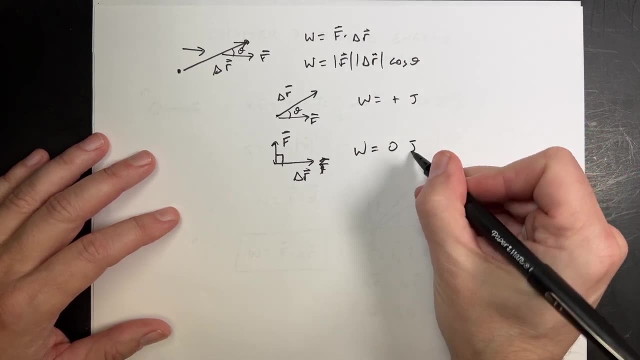 If the angle between those two is 90 degrees, The cosine of 90 is zero, So this would give a zero work. You can have a work of positive joules, You can have a work of zero joules And let's have this case: delta R. 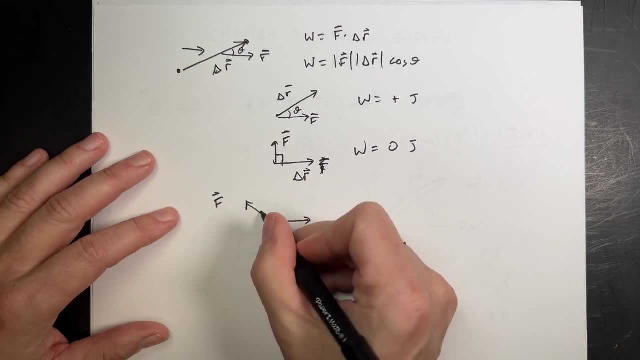 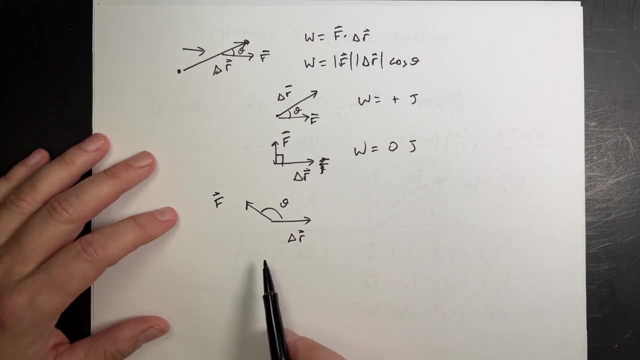 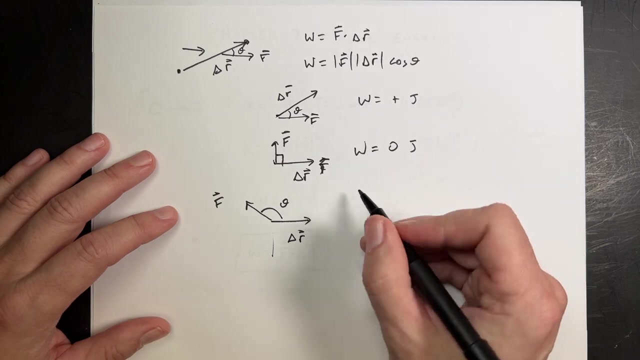 And then F this way, And then here's my angle: If theta is greater than 90 degrees But less than 270.. So anywhere from here to here, Then the force is backwards pushing. You're actually going to get a cosine value that's going to give you negative numbers. 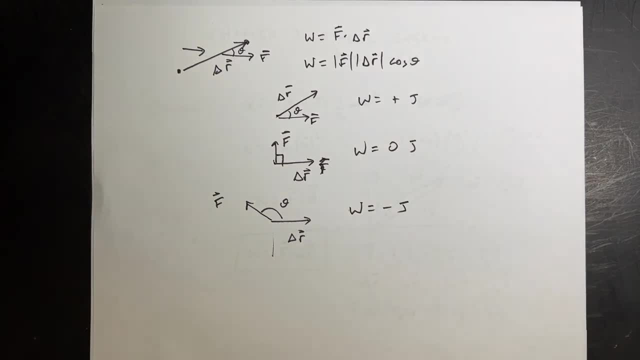 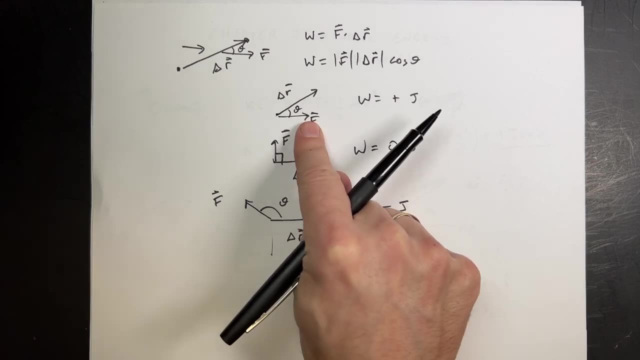 So work would be negative, And that is possible too. And that means that the force decreases the energy of the system. This force doesn't do anything to the energy of the system, And this adds energy to the system. Does that sound good? 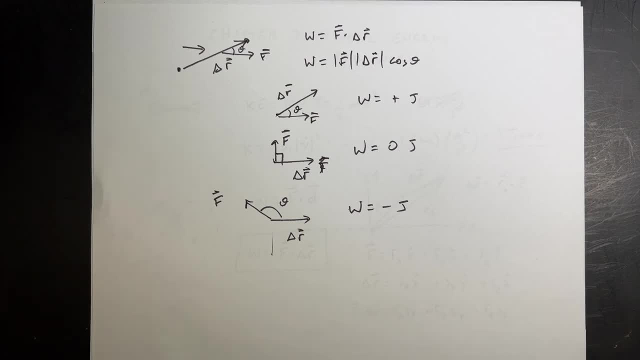 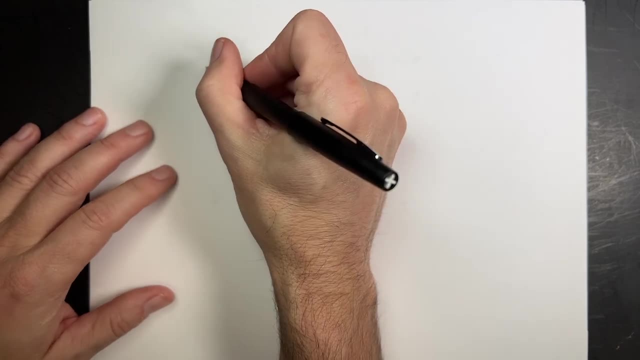 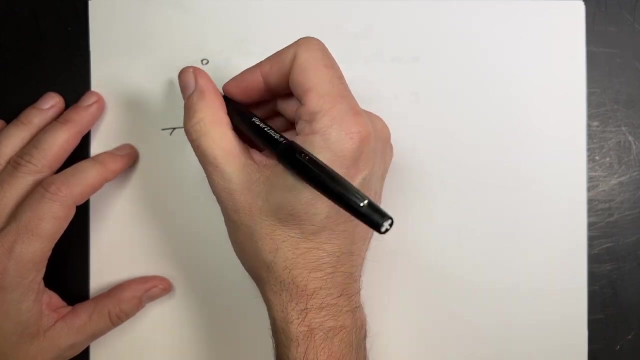 Okay, Next topic: They have a thing about work done by gravity. I don't think it's super useful, But that's fine, We'll do it anyway. So suppose I have this And then I have a ball going from, let's say, Y1.. 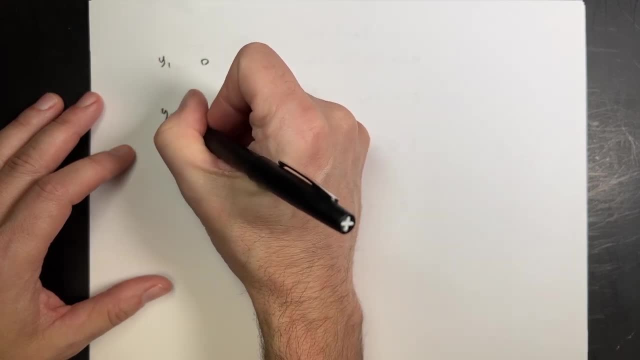 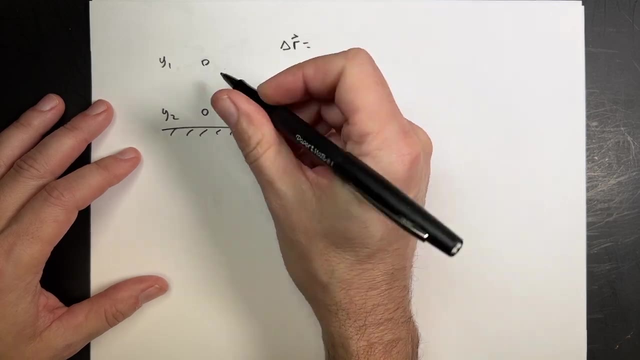 So it's falling To Y2.. And I want to calculate the work done by gravity. Well, the first thing I want to do is calculate delta R. So delta R is going to be the final position minus initial position, So it's going to be zero X hat. 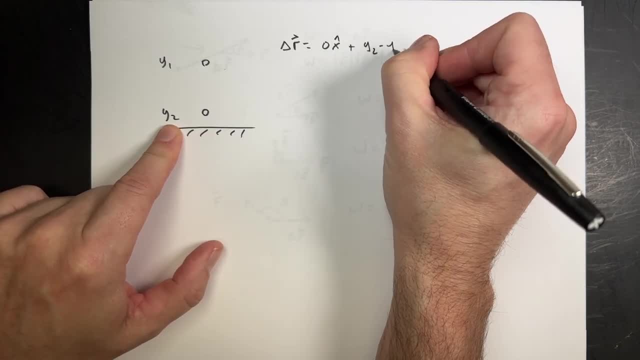 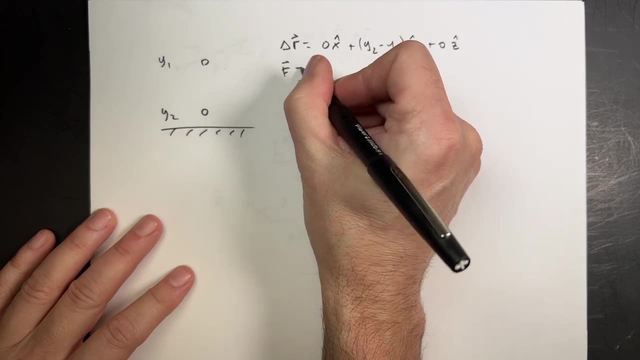 And then this is going to be plus Y2 minus Y1.. Right, Because it's final minus initial Y hat plus zero Z hat. What about the force? F is going to be zero X hat minus Mg Y hat plus zero Z hat. 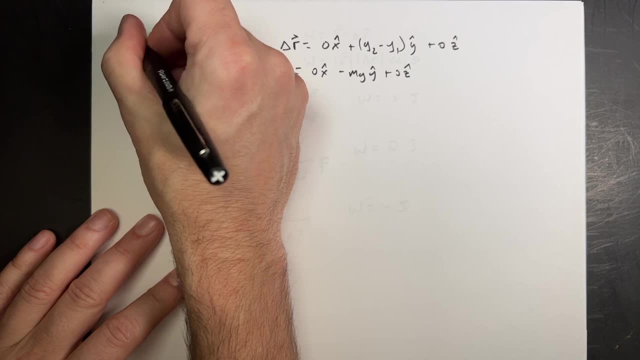 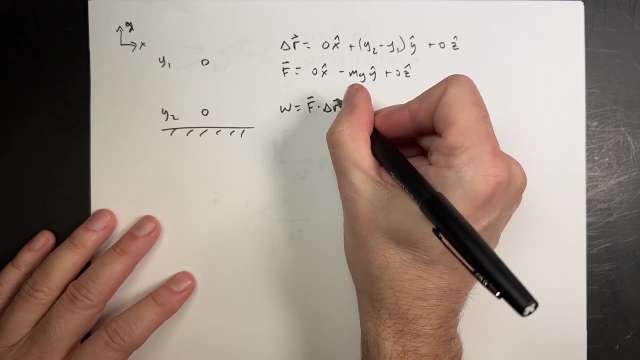 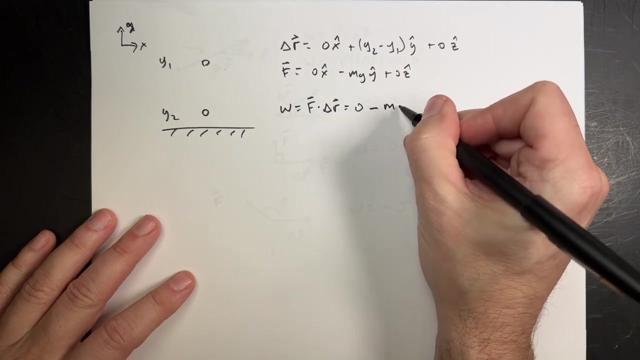 Assuming this normal convention, X, Y, like that. So now if I calculate the work, it's just going to be F dot delta R And that's going to be zero times zero, Zero. This times this is going to be negative Mg times Y2 minus Y1 plus zero. 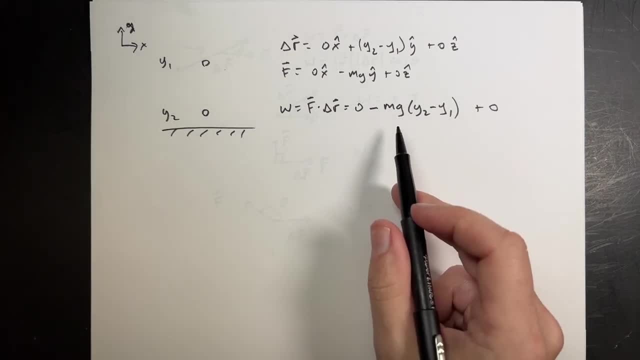 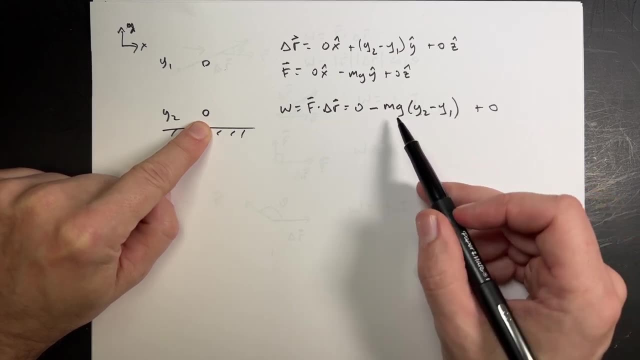 That one is zero times zero. Now is this going to be a positive or negative number? Well, if it's going down, Then Y2 is less than Y1.. So this is going to give me a negative number, And then I have a negative sign over here. 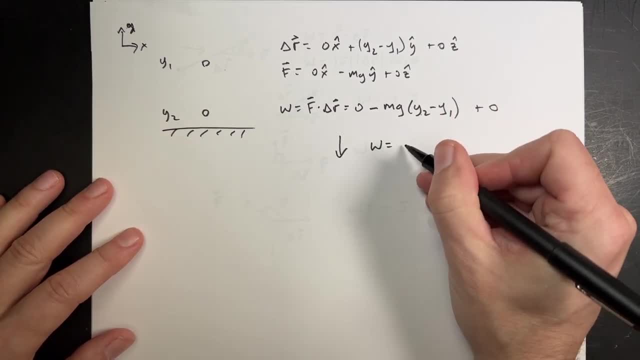 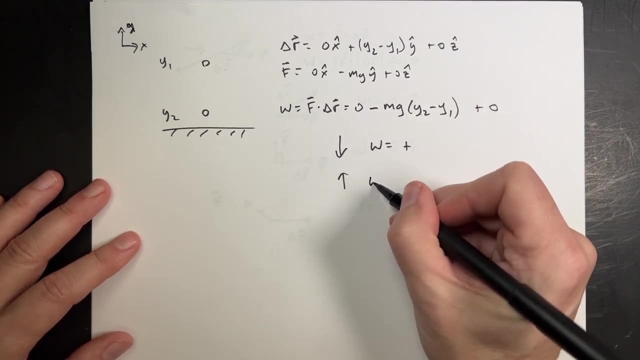 So if I'm going down, Work is positive. If I'm going up, Then Y2 would be greater than Y1. This number would be positive And I have a negative sign, So work would be negative. So if you're going in the same direction as the gravitational field, 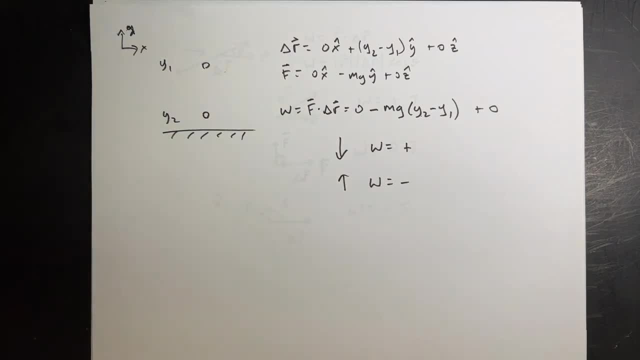 The work done by gravity. Okay, Don't think about the work done by something else. Don't think about potential energy. We haven't talked about potential energy. The work done by gravity Is positive going down, Negative going up. What if I do something like this? 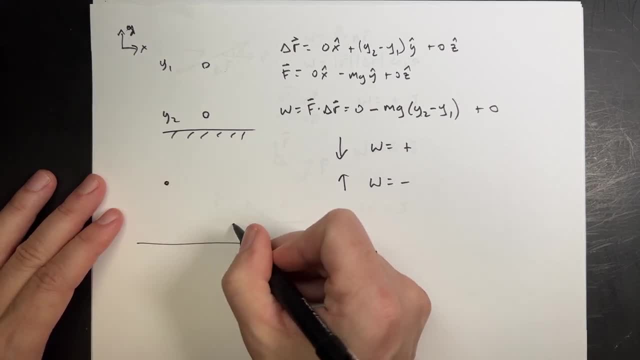 Here's a fun one. I go right here To right there. So this has X1. Y1. This is due in two dimensions. It's a comma To X2. Y2.. Well, in this case, Now I'm going to have a different delta R. 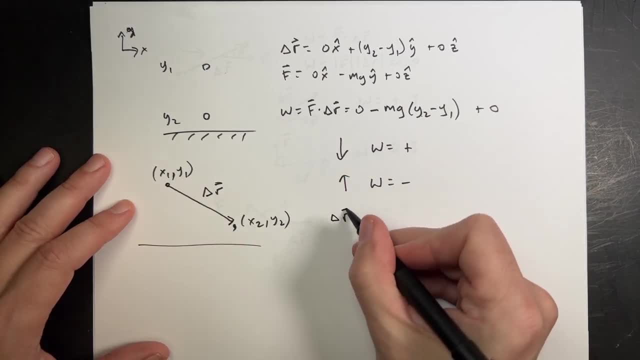 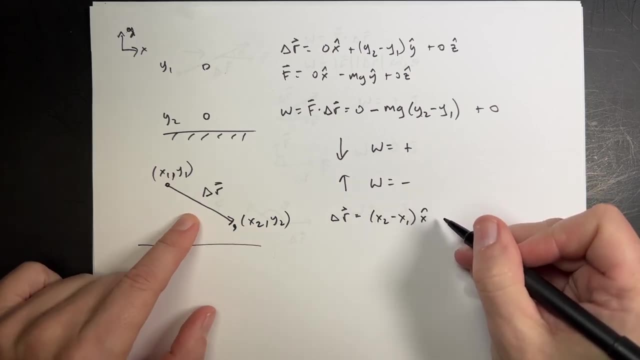 So now I'm going to have delta R- It's going to be the final position- X2. Minus X1. X hat, And then Plus Y2. Minus Y1. Y hat Plus zero Z hat. 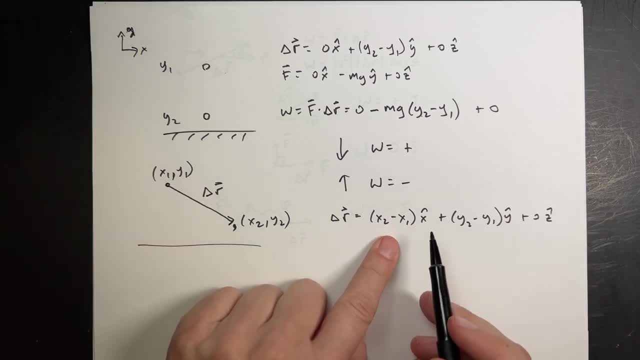 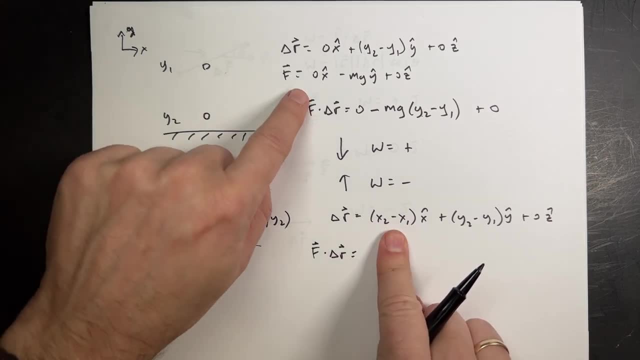 If I take this And dot it with this F dot, delta, R, Notice that This is multiplied by zero, So it's just going to be zero. And then I do this again, I get minus M, G, Y2.. 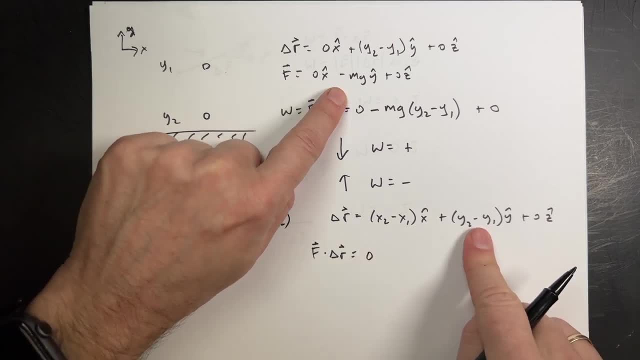 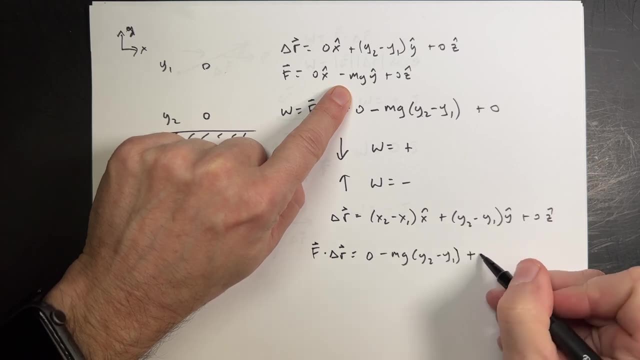 Minus Y1. And then X2.. Minus X1. X hat, And then Plus Y2.. Minus Y1. Y hat, And then Plus zero. So I actually get the same thing, And that's one of the things you'll notice is that 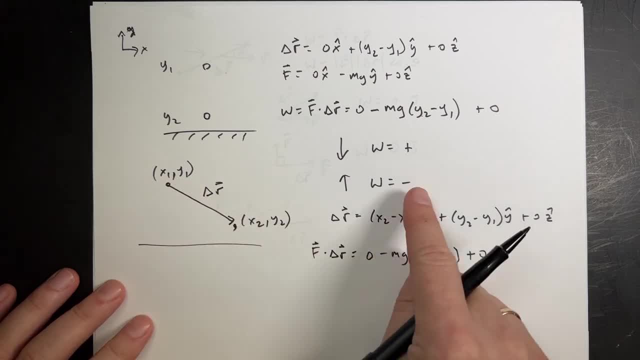 Horizontal motion doesn't do anything. If I'm only moving in the X direction, Because the component of force in the X direction is zero For gravity, Then I'd get zero work. Okay, So in this case Only the vertical stuff matters. 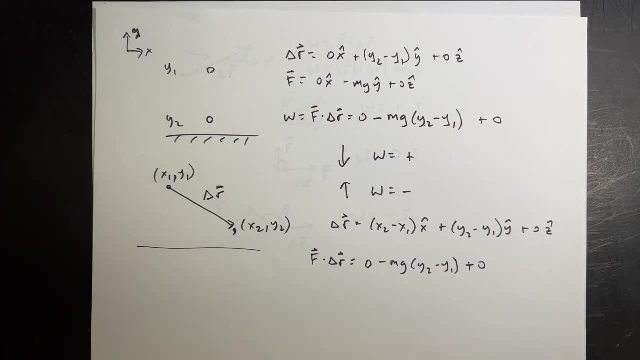 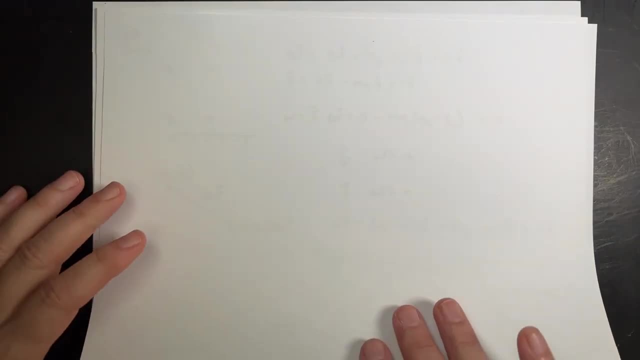 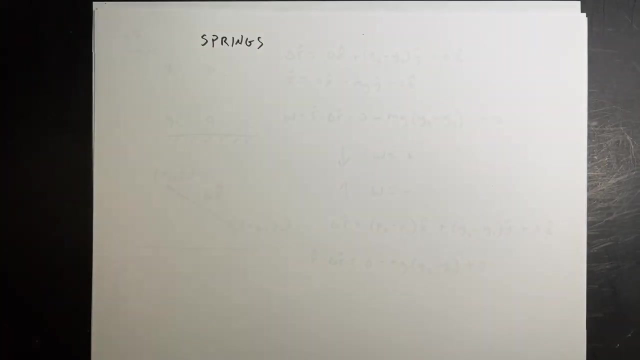 And we'll see that's really important later When we get to potential energy. Okay, Next Springs. So springs are super useful in physics Because It turns out that we can approximate a lot of interactions as though it were just a spring. 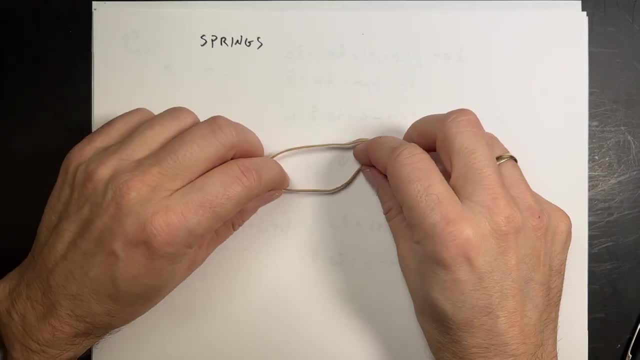 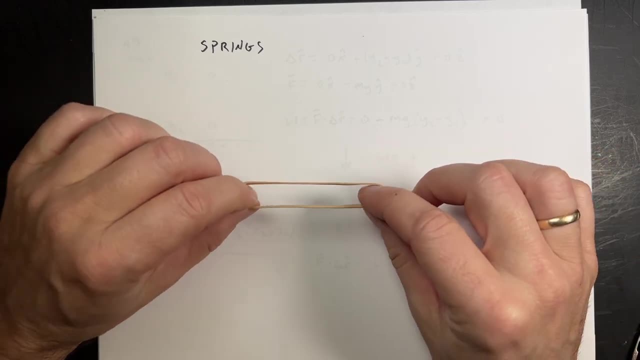 Here's one that's really nice. This is a rubber band. It's not a spring, But it's kind of springy And it behaves a lot like a spring in some situations And that makes it fun. But in general, An ideal spring. 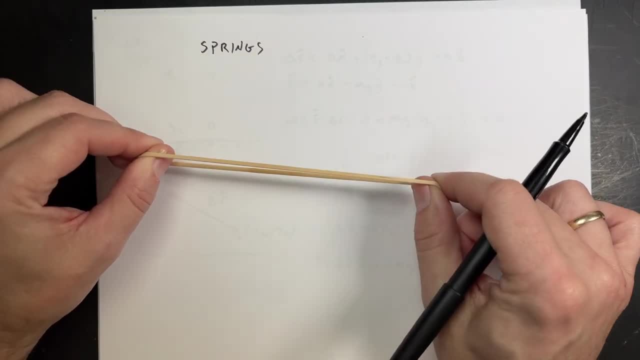 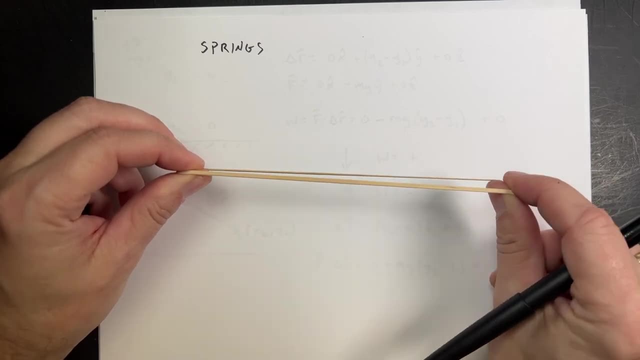 The more you stretch it. If I stretch it that way, It's going to pull back that way. So, And the If I double the stretch, It doubles the force. So that's one of the things. It's a non-constant force. 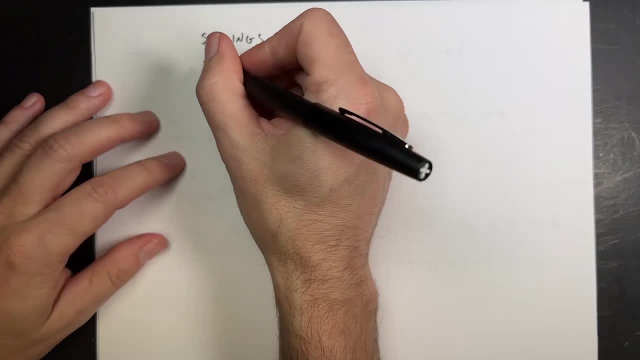 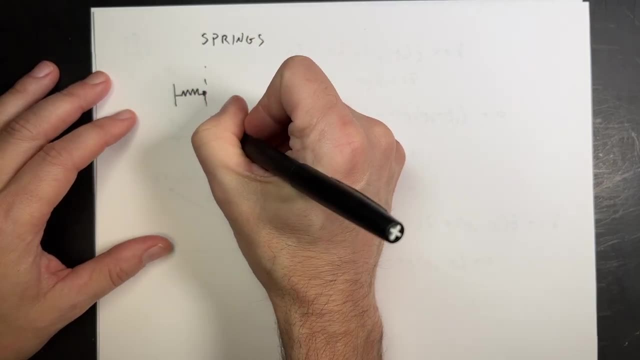 And in the X direction. This is the way the book writes it. It says We can draw it like this: So say, I have a spring right there, And this is at X equals zero. And then I stretch it: There's X equals zero. 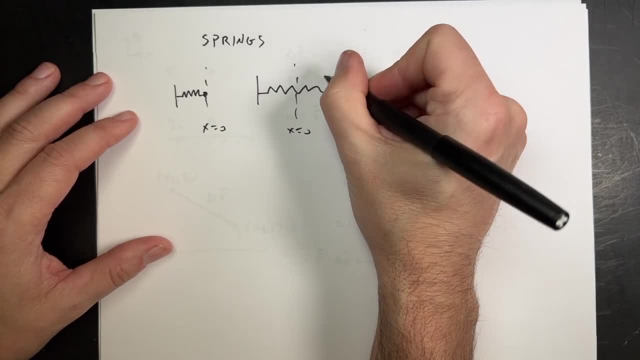 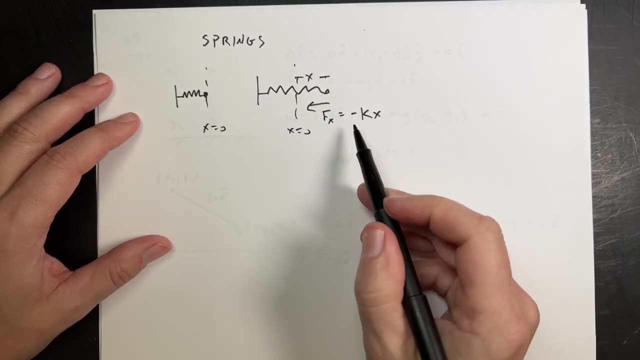 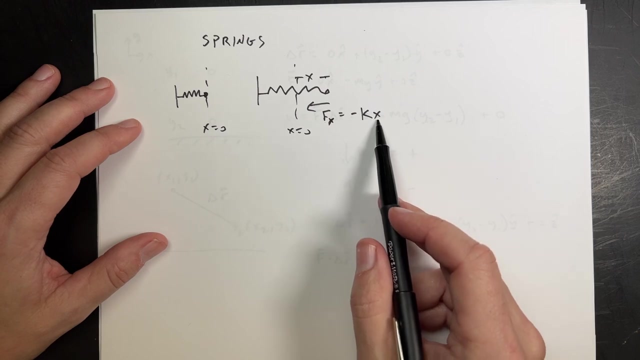 X equals zero And this is X. Then the force Fx Is going to be equal to negative Kx, So this is one way to write it. I don't think this is the best way. This says that The force is proportional to the position. 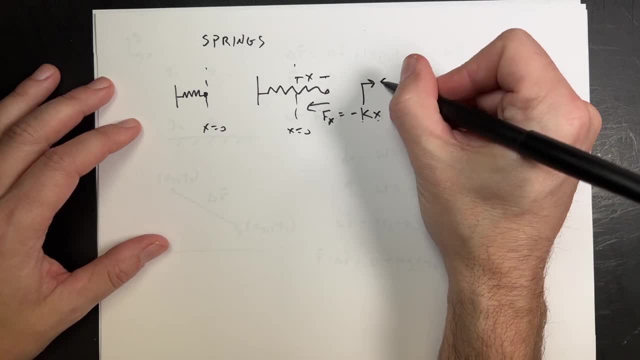 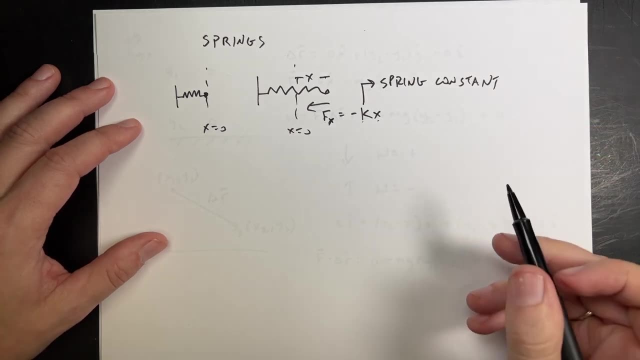 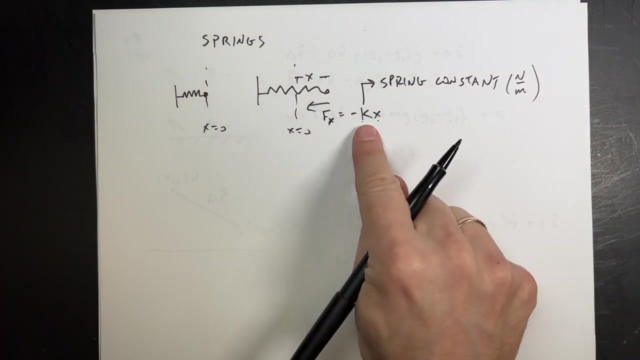 K is called the spring constant. It's basically how stiff the spring is. It's basically How stiff the spring is And it has units of newtons per meter, So a stiffer spring, If you stretch it, the same amount As a weaker spring. 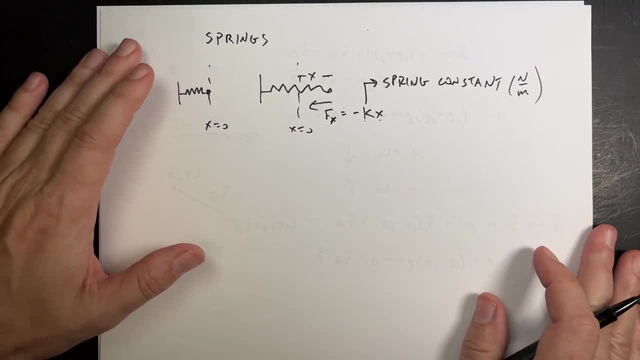 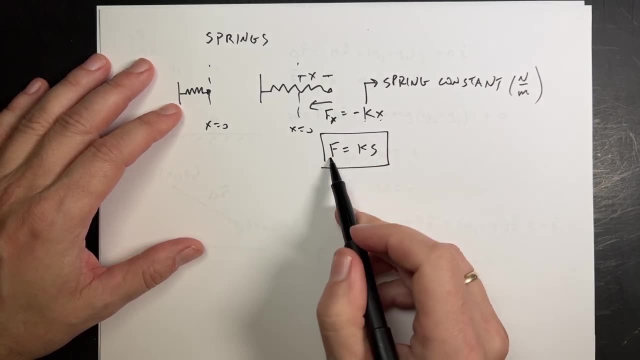 Will have a greater force. Now I like to use. There's two ways I like to write this. I prefer to write This is just F, Equals K, S, And not put the negative sign, Because this is the magnitude. 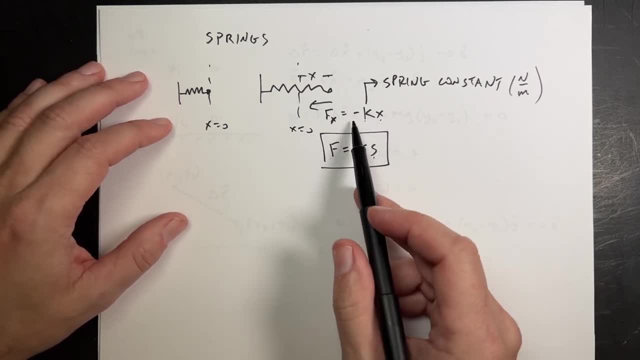 And that's a magnitude. And so You have to know the direction. Right, If you want to, If this is not wrong. I just don't like it that way. The other thing is: What if? What if it doesn't start at? 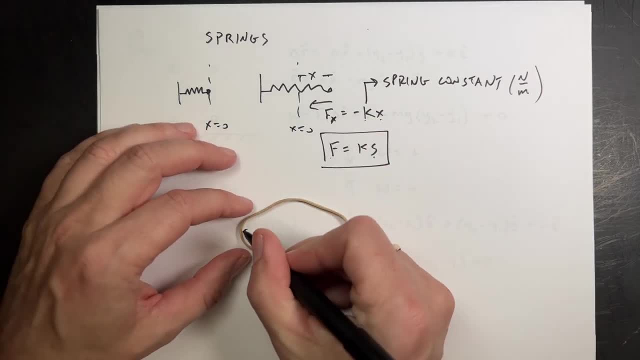 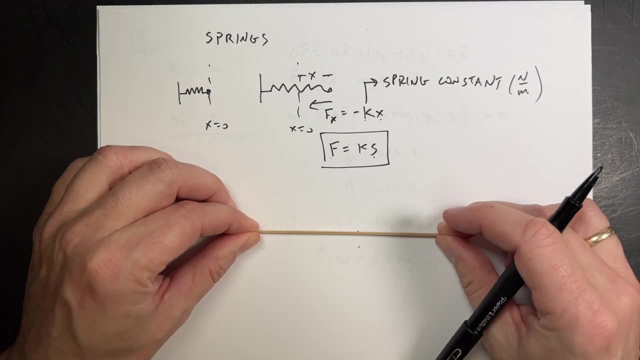 X equals zero. That's a little bit more difficult, I mean. So Imagine This is my origin, And then I start right here. See, I have a rubber band And then I stretch it. In that case, Let's say: 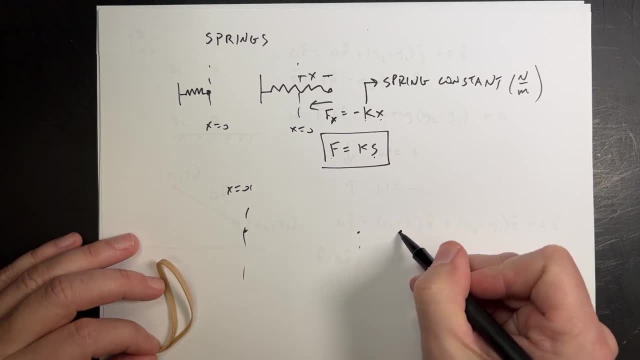 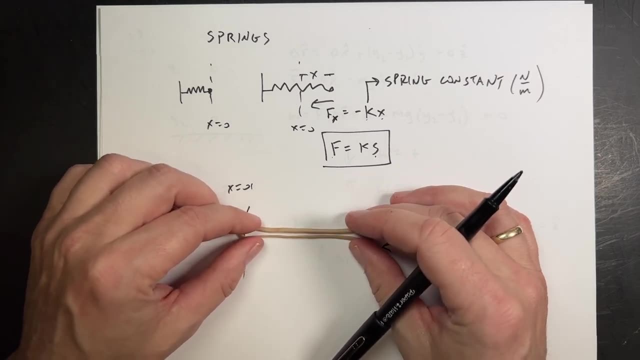 This is: X equals zero, And then I stretch it over to here. Obviously, The force is going to be Back that way, But how would I calculate that? One of the things you need Is this Unstretched length. 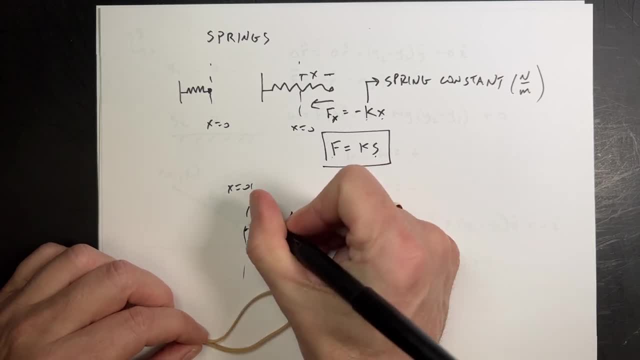 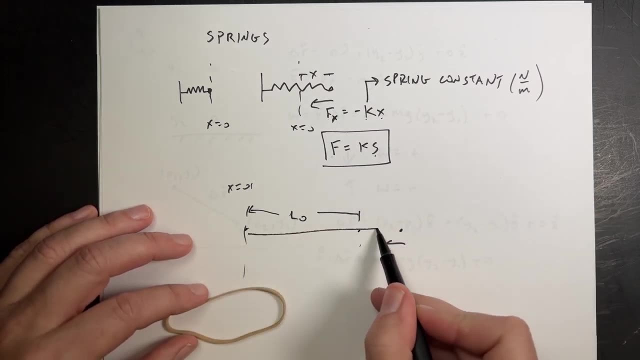 Let's call that L zero, And this is the way My favorite technique, My favorite textbook Does it, So I like to do it this way. In that case, I can calculate This vector L. I'll call the length. 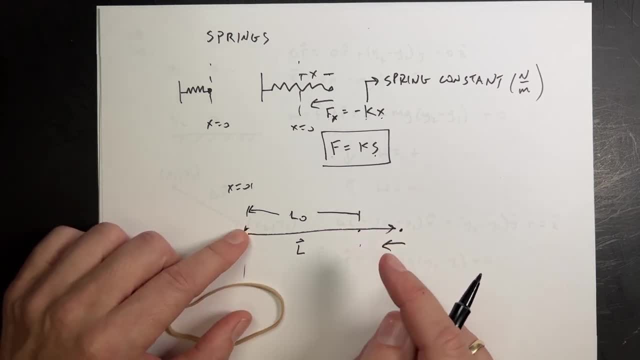 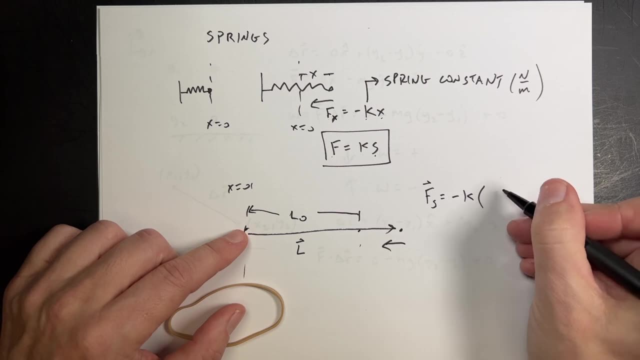 Of the rubber band L From where it starts To where it ends And it's a vector And with that I can say The spring force Fs Is going to be Negative K Times, The magnitude. 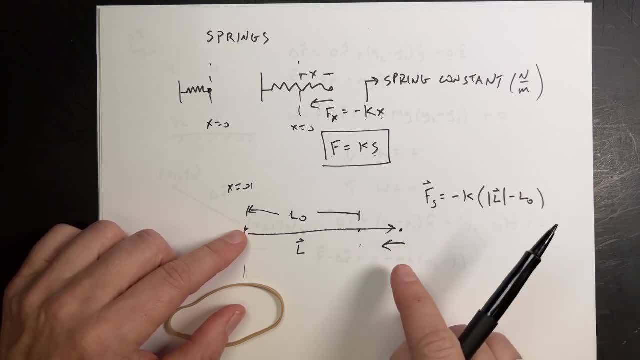 Of L Minus L zero. But see, Then, If I do that, Then I'll get this back As a vector. I'm going to multiply By L Hat, So L Hat Is a unit vector. 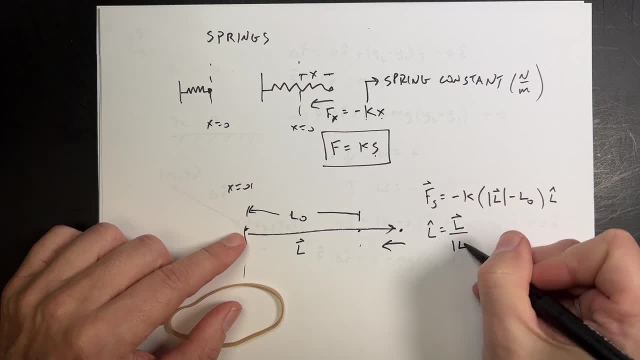 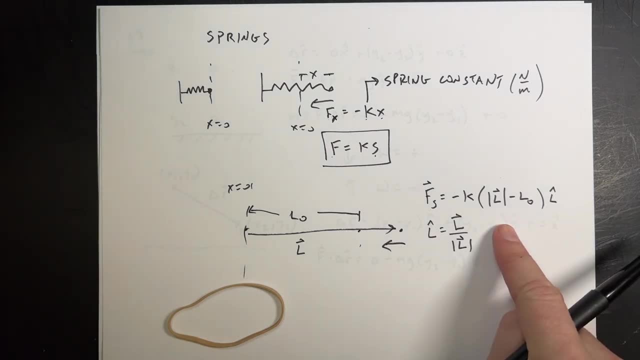 In the direction Of L. So L Hat Is going to be The Vector L Divided By the Magnitude Of the Vector L. This Looks Cumbersome And a lot of times. 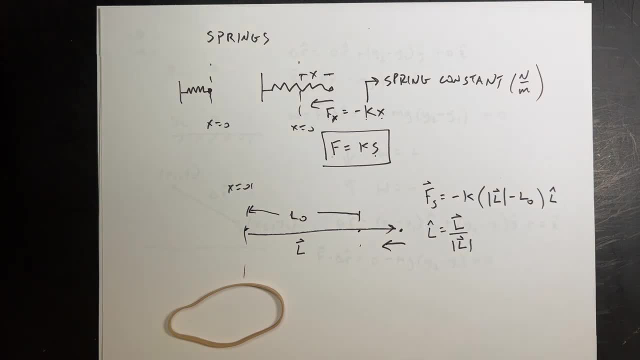 You can avoid this, But I'm not doing that In the video, But I think It's an important thing To do So, So Make sure If you're interested To look at that. It's the way. 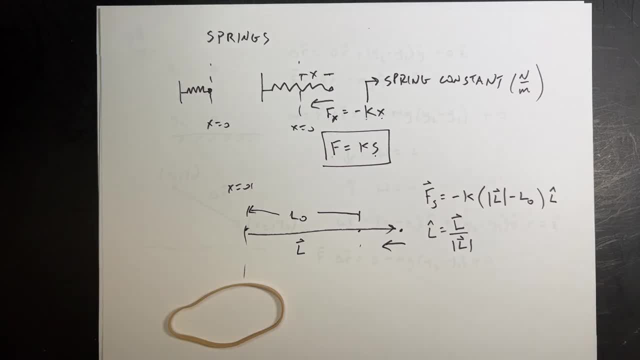 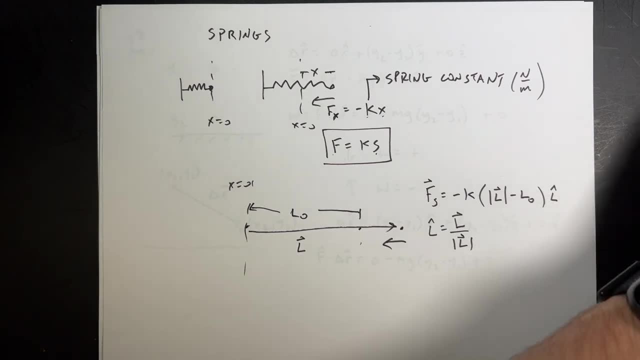 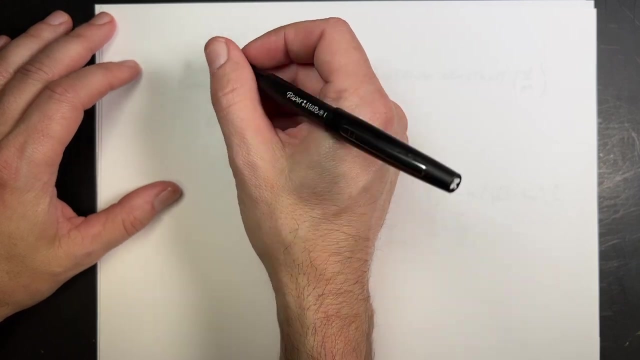 We do Physics Now. Anyways, This idea Of a numerical Calculation, But This Allows You To Calculate The Force As A vector. So Suppose I have A spring And 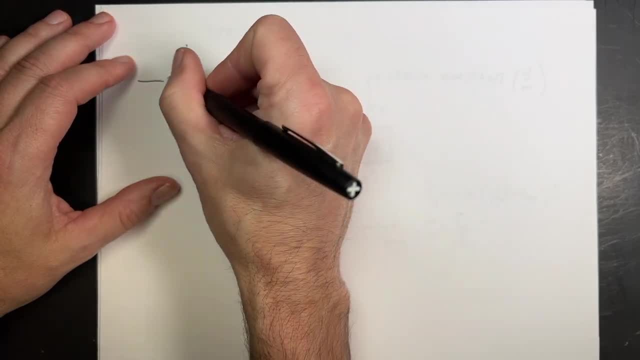 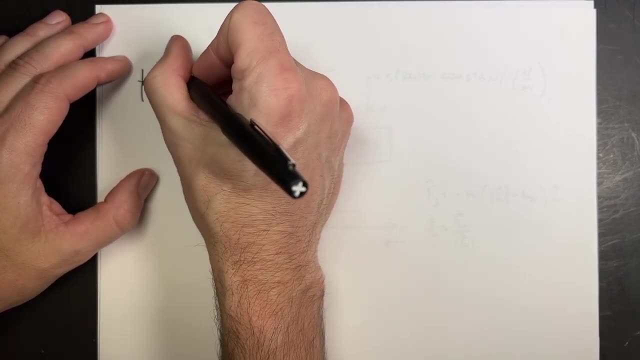 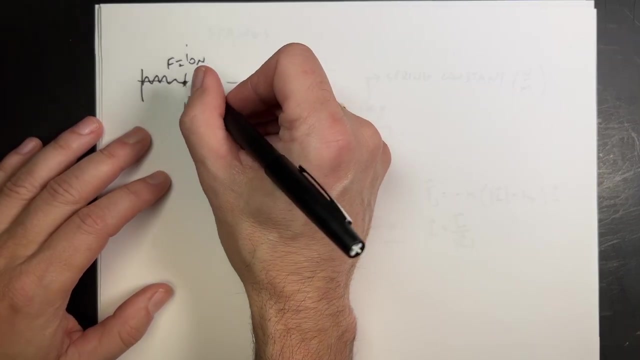 This Is At X Equals Zero And Then It's Attached Over Here. This Is Unstretched, So F Equals Zero Here And I'm Using Just 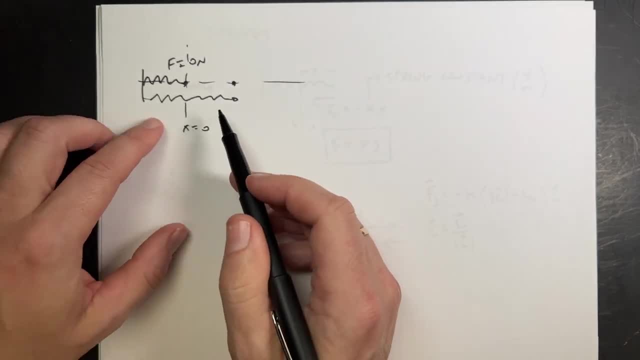 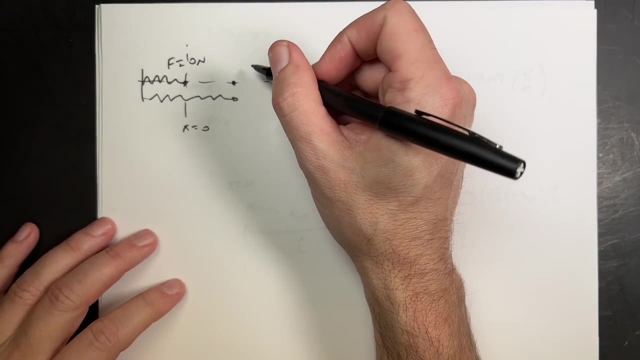 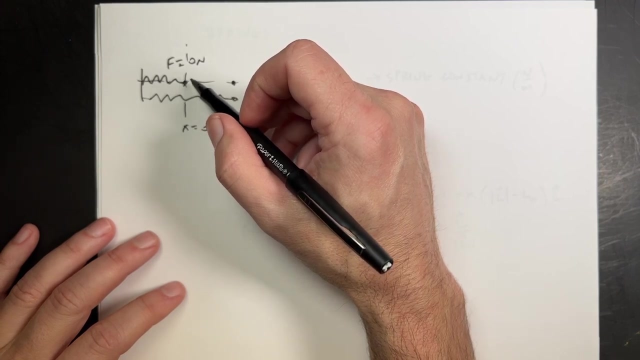 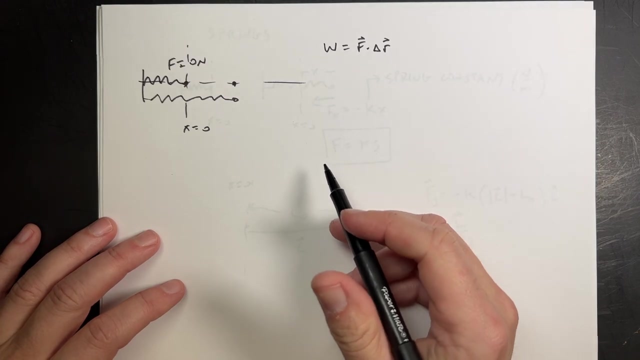 This And I Want To Calculate The Work Done By The Spring Over That Distance. Well, I Have. I Have A Problem, Because Here's My 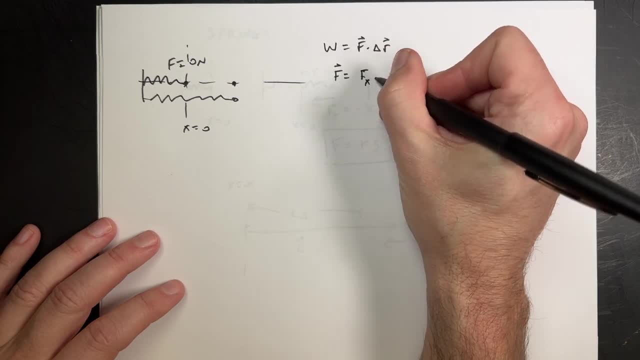 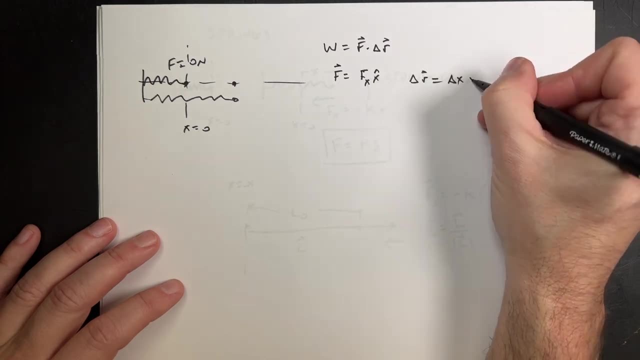 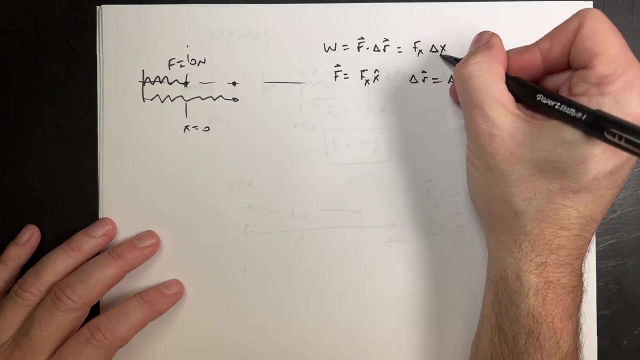 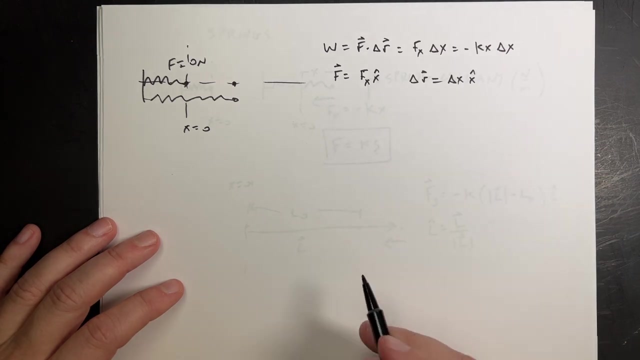 Definition Of A Constant: F X, X Hat Doesn't Have Any Y Components And I Can Write Delta R As Delta X, X Hat. So 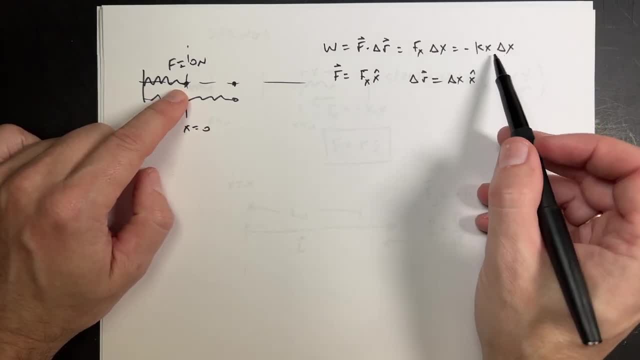 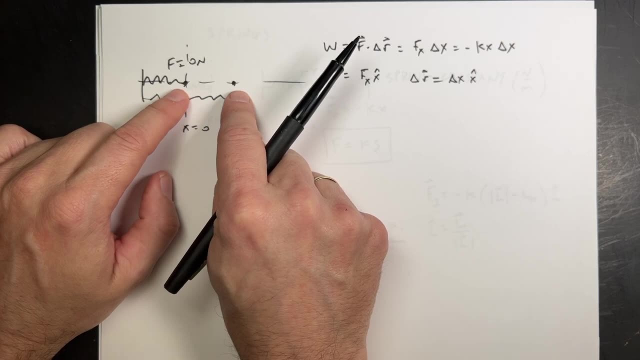 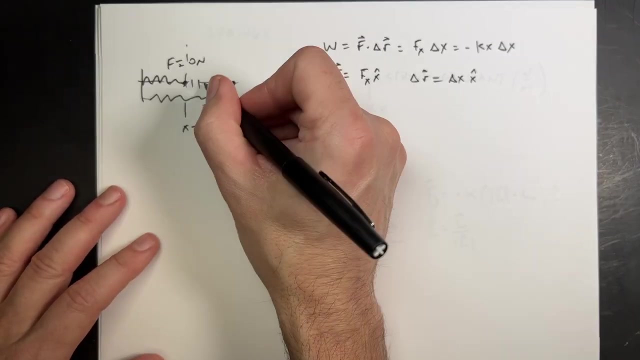 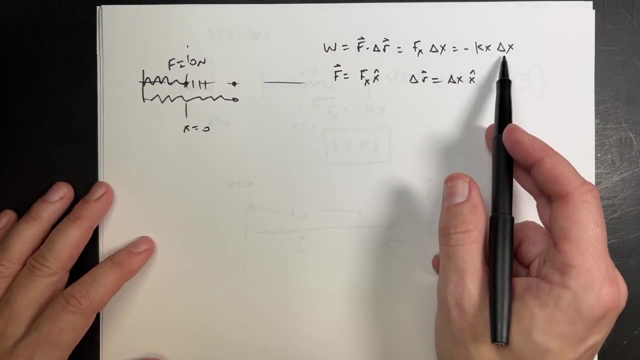 F, Dot, Delta R. This Is Just Go From Here To There In A Simple Way And In Fact, I Need To Break This Into Tiny. 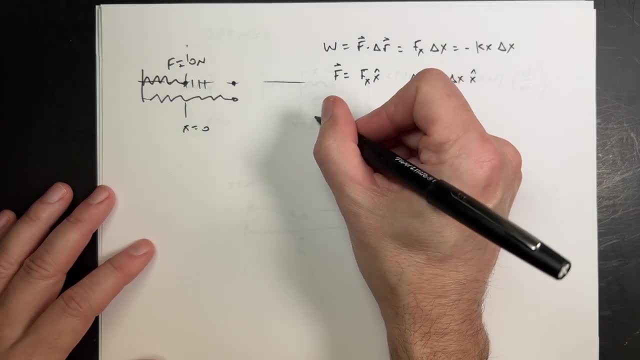 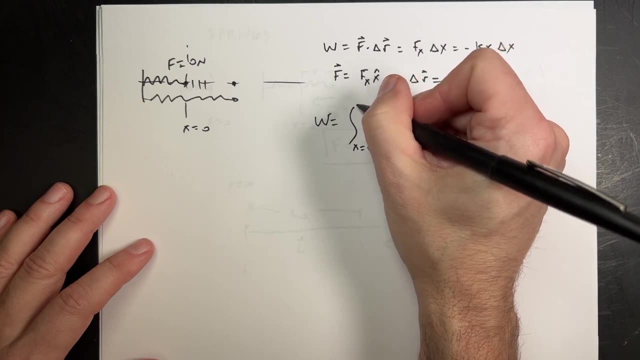 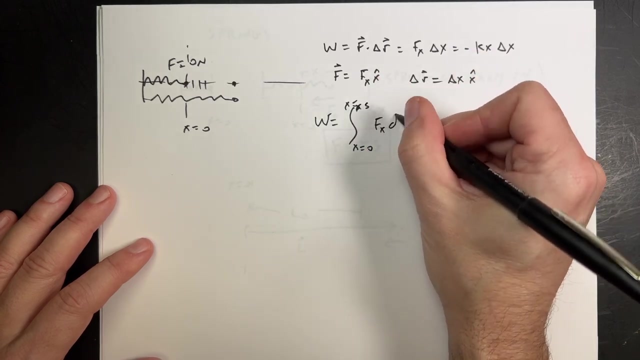 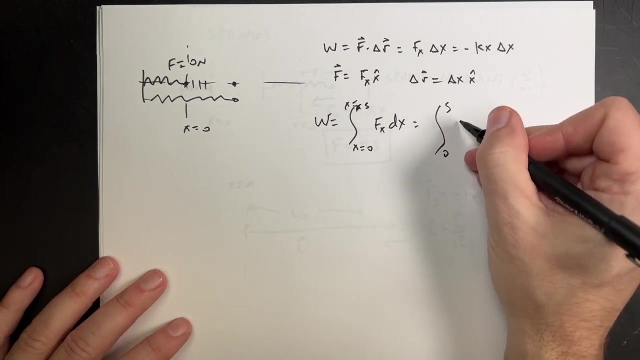 Tiny, Tiny Steps. If I Just Go A Little To X, Final A Call, Let's Call S To X. Equals S Of F X D. 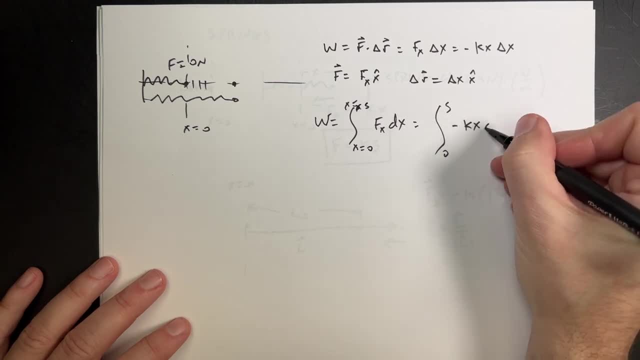 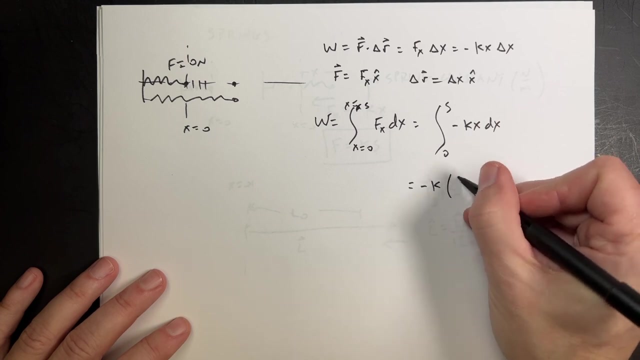 X. Right, I'm Going To Let That Delta X Go Zero And I have x to the 1, I raise that by 1 power and divide that by that 1 power, So I get 1 half x. 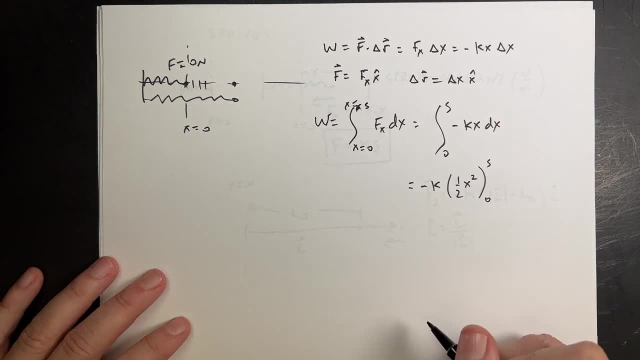 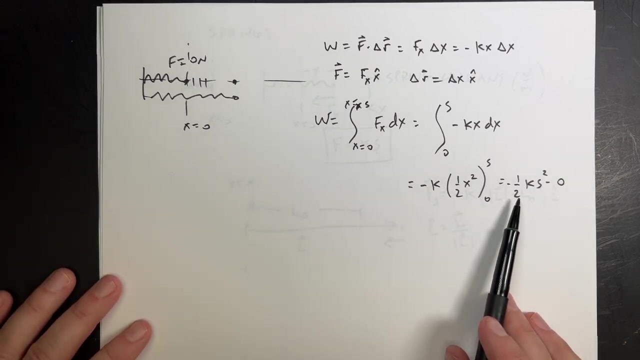 squared from 0 to s- Now I'll just plug that in- I get negative 1 half k s squared minus 0. So the work done by the spring is this negative value And in fact we can generalize this to the. 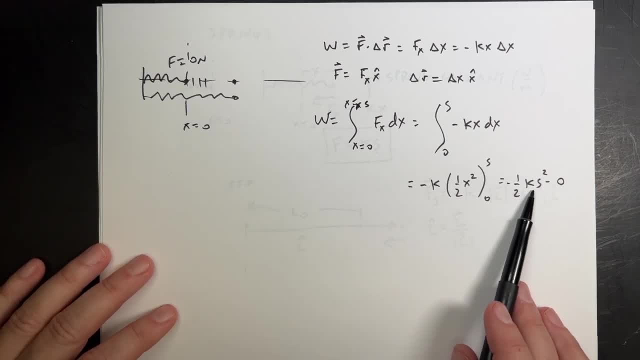 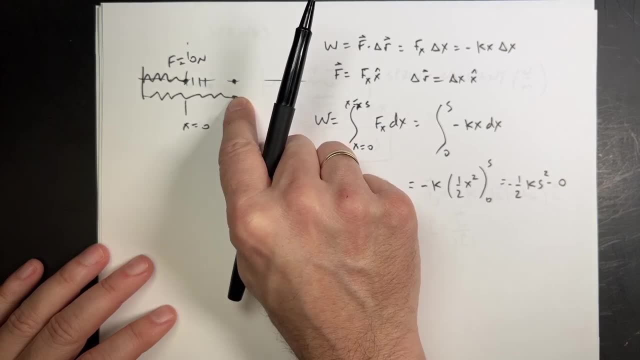 uh, yeah, that's, that's what we want. The work done by the spring is negative 1 half k s squared for if you're stretching it, Um, if it's going the other way, if you, if you have it stretched. 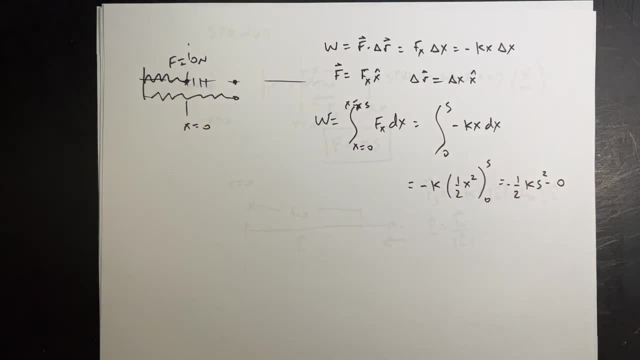 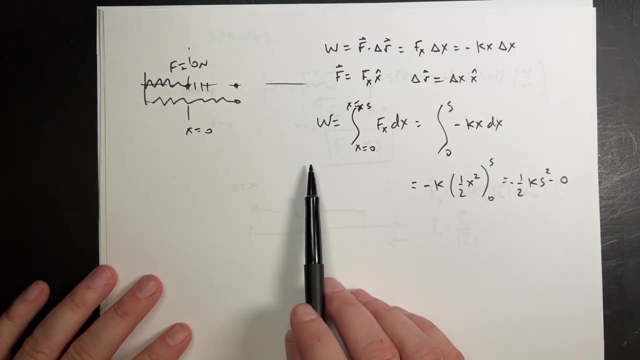 already and you let it go back the other way. you just switch these limits of integration. you get a positive number. but that's the work done by the spring And- this is the important thing- the work done by a variable force. This works for any force that's not constant. 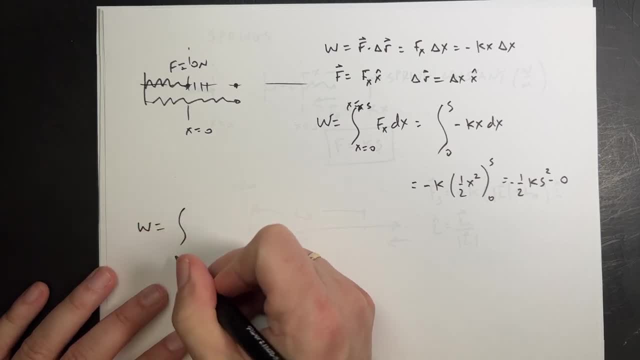 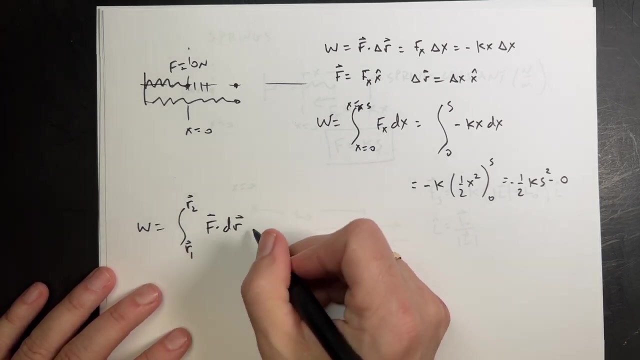 I like to write it in general work: equals the integral from r1 vector to r2 vector of f dot dr, where this is really going to break into. line integrals can get a little tricky but nothing complicated in this course. Uh, this can break into the integral from: 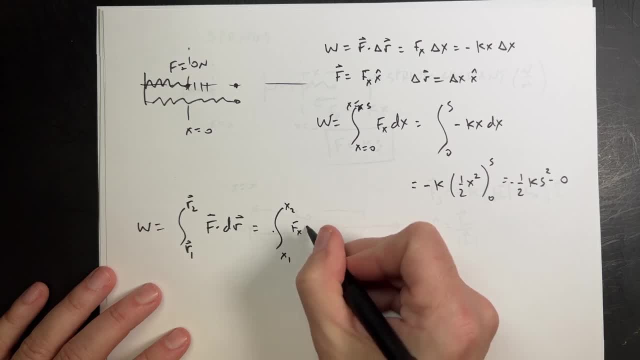 x1 to x2, fx dx, plus the integral from xy1 to y2, fy dy, plus the integral from z1 to z2, fx dy, z dz. So you have to know the function of f and how it changes in both the xy and z direction. 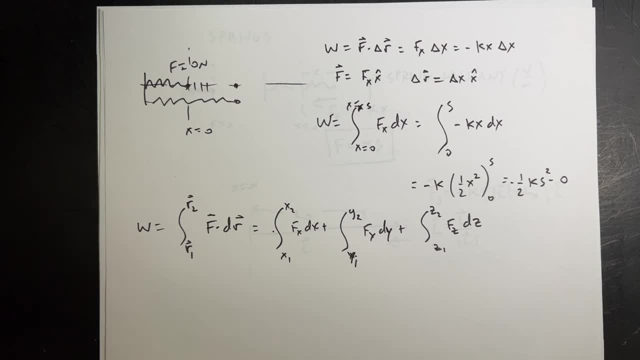 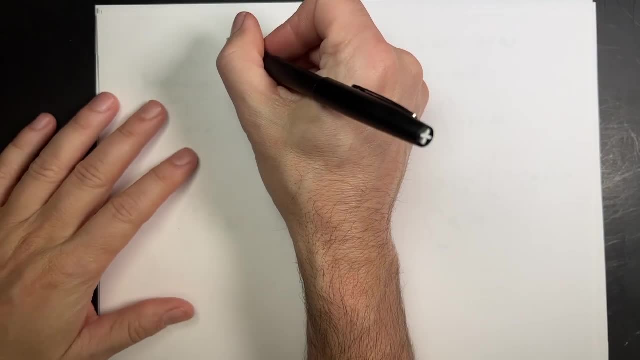 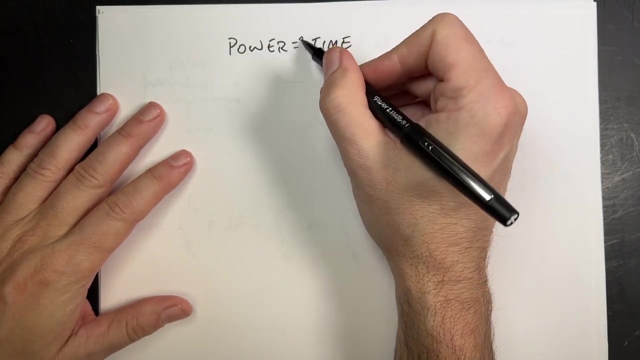 and you can calculate that, And we're going to do that in the next chapter too. We're going to do some practice with that, Okay. One last thing is power. Power is equal to time. No, that's a joke, It's actually not true. right Time is power. No, wait, money is power, Money. 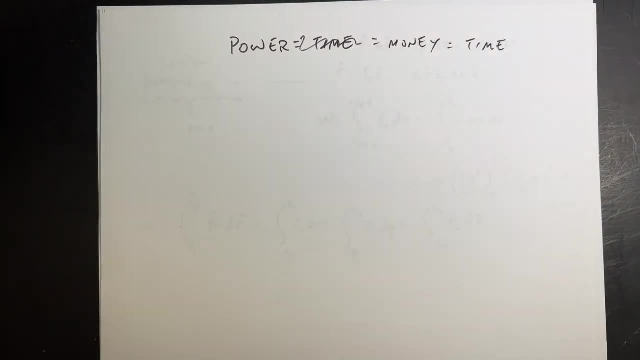 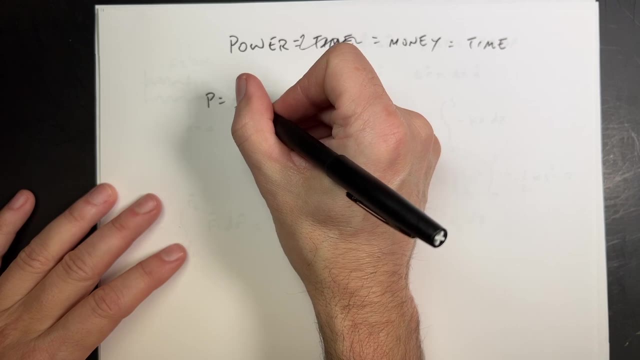 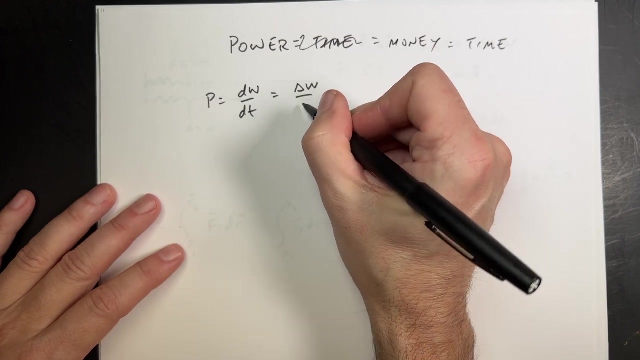 Time is money, So time is power. I was right, That's an old joke. Okay, So we define power as the rate of change of work, So it's dw, dt, And a lot of times we can write this as delta w over delta t, And this has units of joules per second. 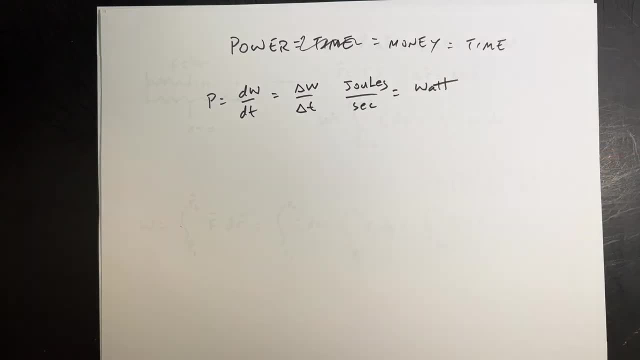 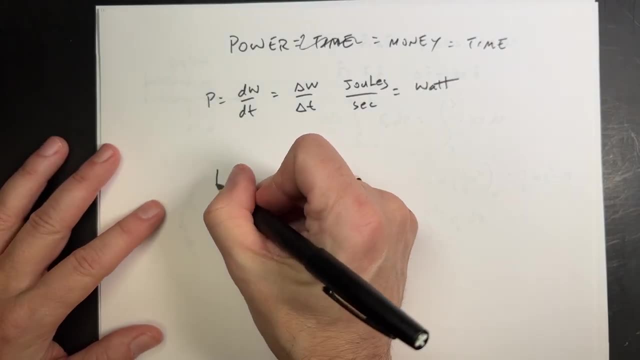 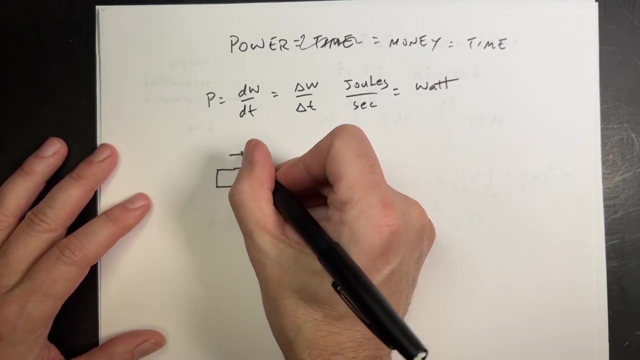 And that's equal to a watt. So it's how fast, How fast you do work. One of the common things that you look at is: suppose, one of the examples, suppose- and it doesn't come up that much- Suppose I have a force pushing on here and this is moving with some velocity. v. 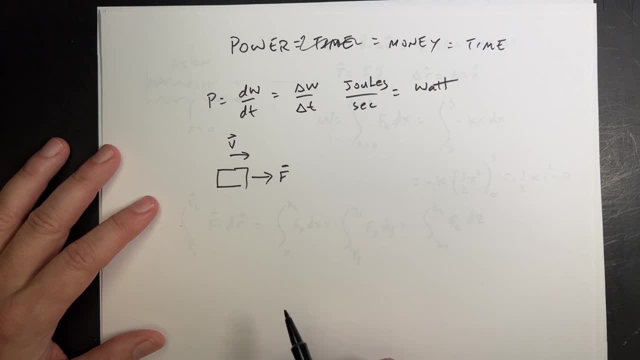 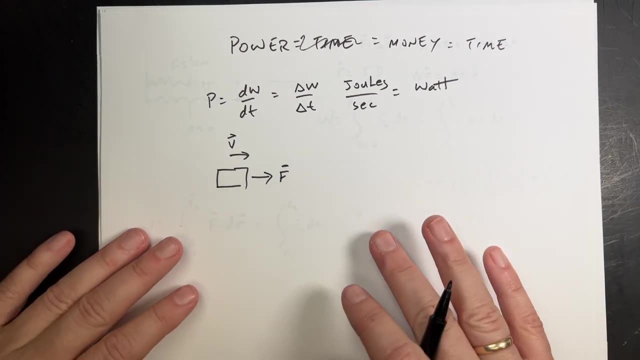 And we don't need to worry about the direction. that much, Suppose it does that. And oh, did I ever write down the work? kinetic energy theorem. This is the whole point. Well, I'll put it over here. Work is the change. 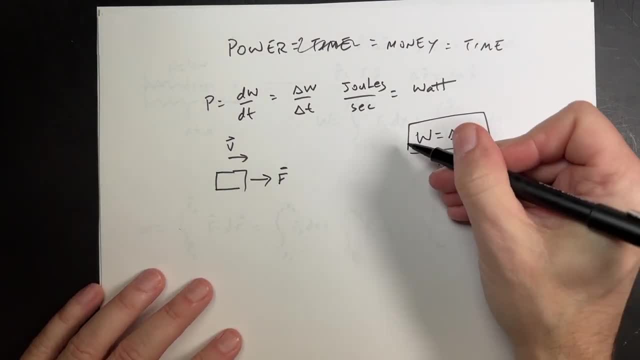 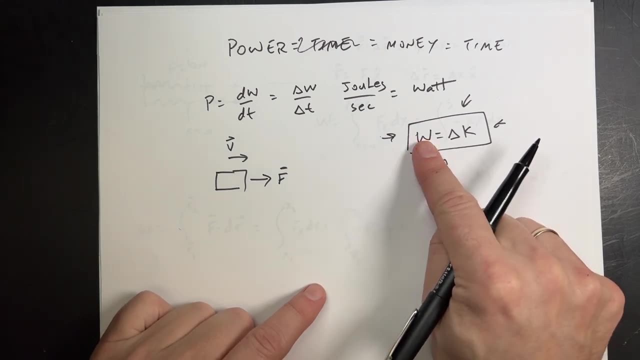 And kinetic energy. That's like a big deal, Big deal. Right, It's a big deal. This says that if I have some system, the work changes the energy of the system And at this point, the only energy that we have is kinetic energy. 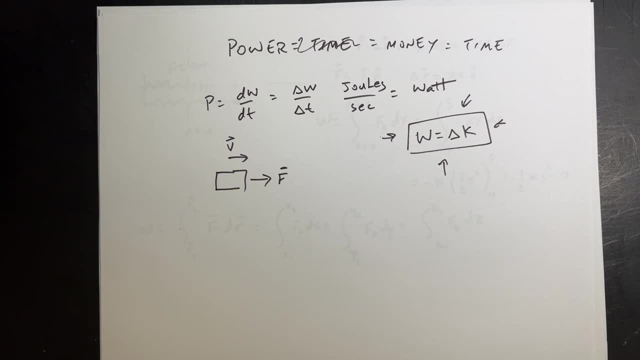 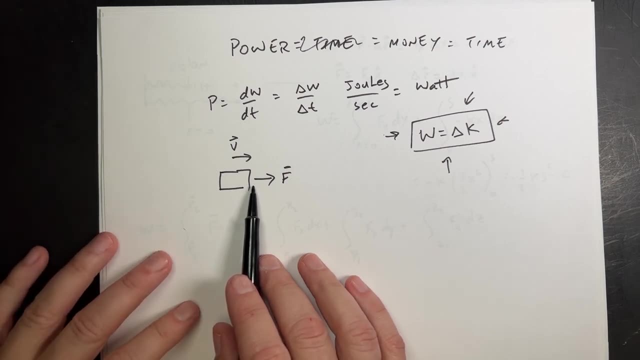 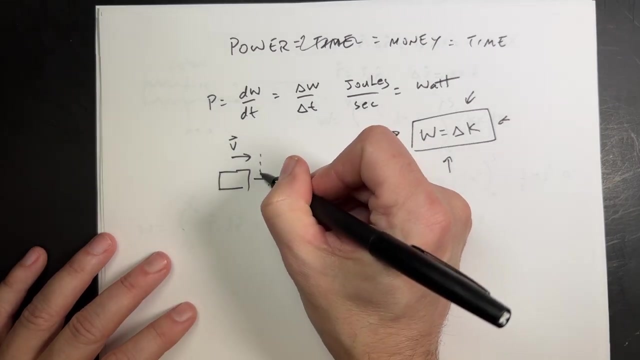 Okay, So that's how we connect these two. That's work and kinetic energy. That's the name of the chapter. So suppose I'm pushing on this with some force and it's moving with some velocity. v Now Let's just take a super, super, super short time interval such that it moves some distance. 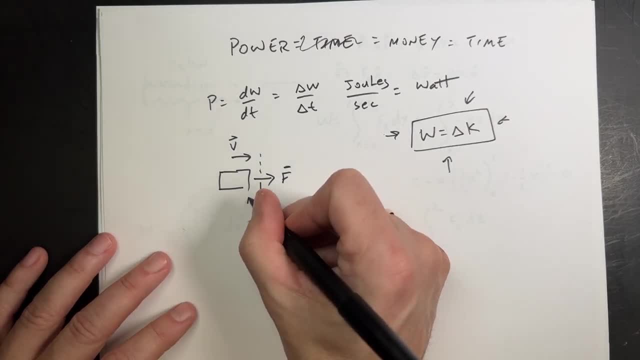 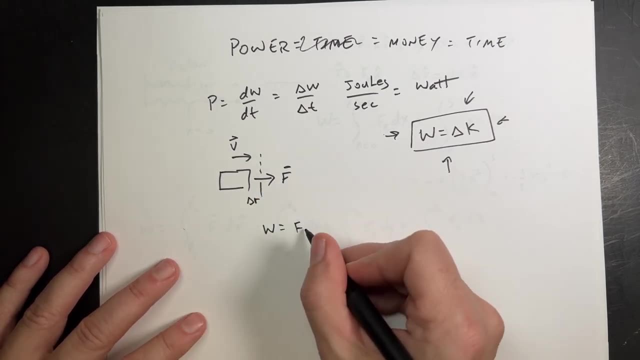 and the velocity doesn't really change that much. So we can call this delta r as the distance. So now I can calculate the work. Work is going to be. it's the same direction f. No, it doesn't have to be. 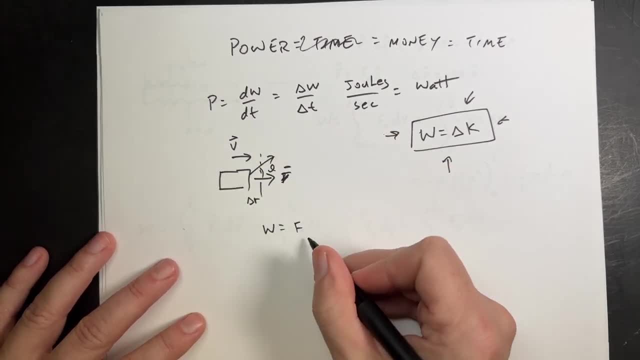 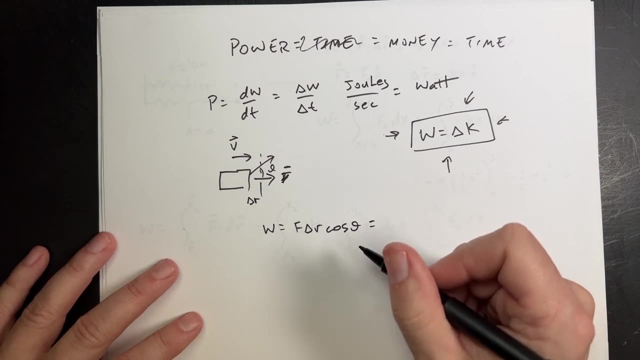 So it's going to be. let's say, f is that way And this is the angle theta. So it's going to be f, delta, r, cosine theta. That's the work done And that's going to be equal to the change in. 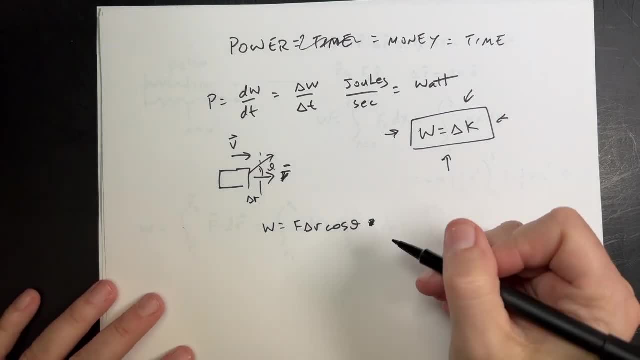 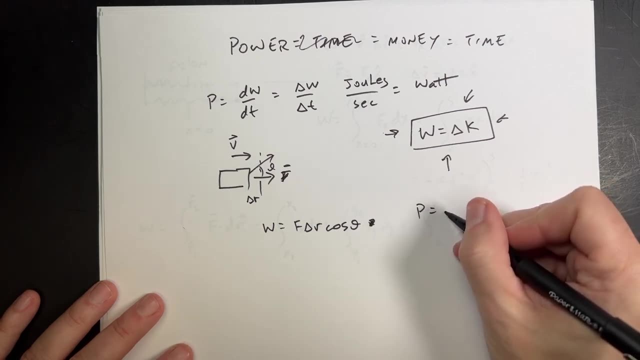 No, that's fine, That's all I want. So now I want to know the power this force does for that object. So I can say power is the change in work over the change in time. So if I take this as my change in work: f, delta, r, cosine, theta and I divide by delta t. 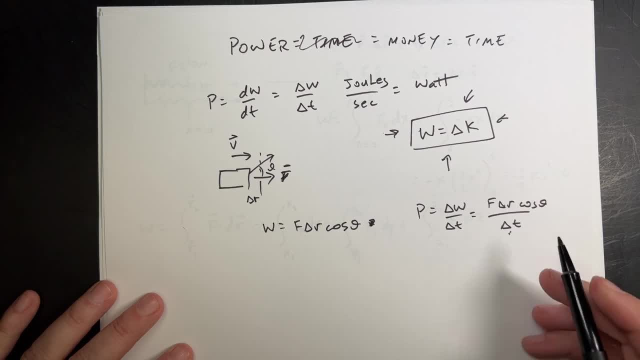 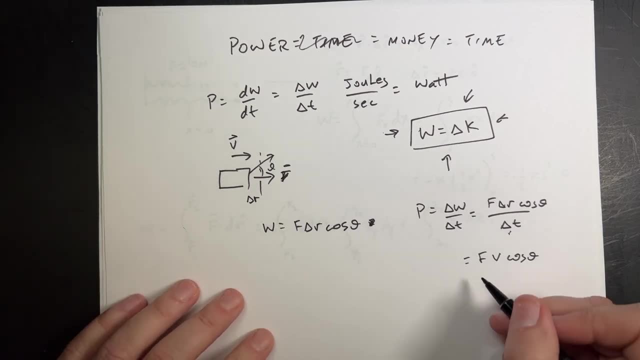 I have delta r over delta t And delta r over delta t is the velocity. So I get f v cosine theta. And just as a check, let's check. this has units of newtons. A newton is a kilogram meter per second squared. 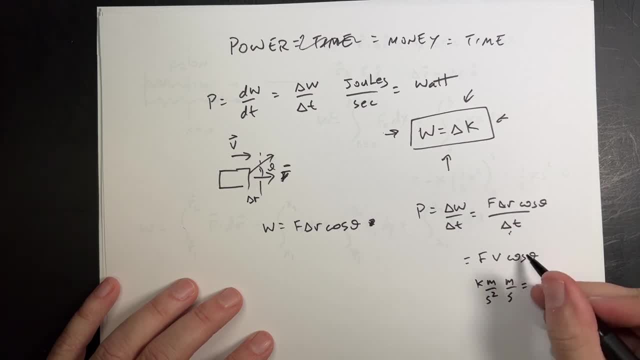 And then I have meters per second, And then that has no units. Cosine has no units. So I get kilogram meters squared per second, squared per second. So this has units of joules, That has units of seconds. So joule per second is indeed a watt.